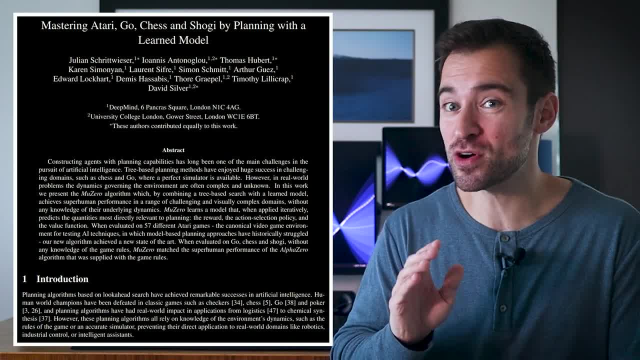 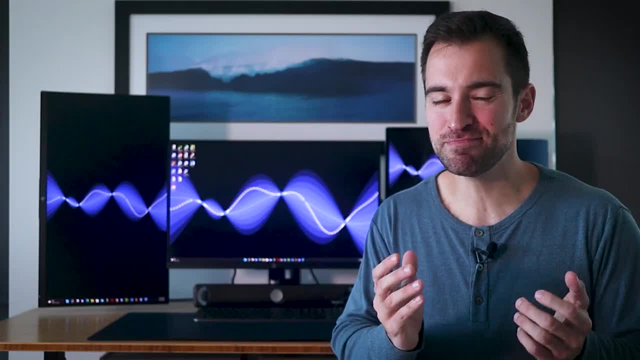 but on a much more diverse set of tasks like playing Go or Atari games, all without being told the rules of the game. As impressive as that is, that never really got me to study the subject. It just didn't seem like a relevant skill set. But that perspective changed when I saw it used. 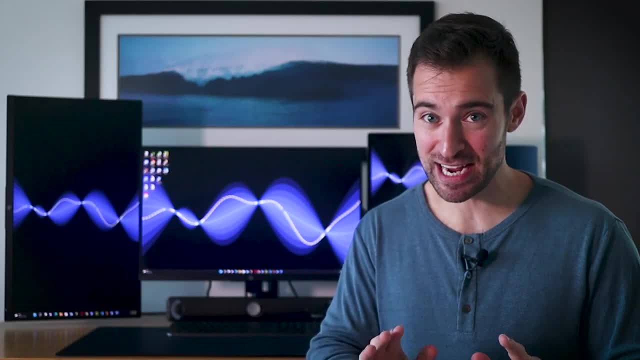 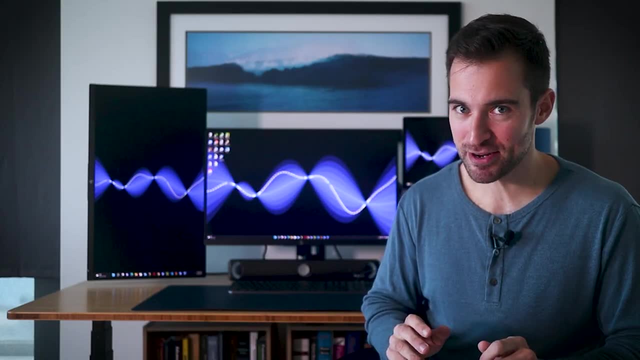 in production at Lyft where I work, having a real, tangible dollar impact right next to me. That got my attention So I looked into it and learned a lot about it and left with a pretty strong conviction. It's a speculation, but from what I know now, I believe that over the next 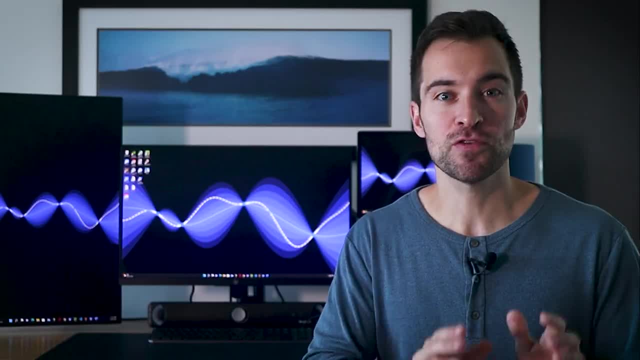 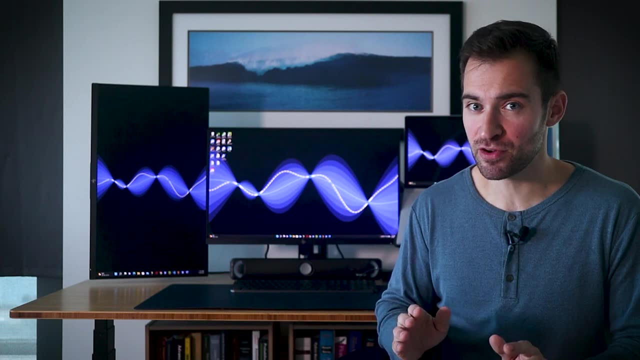 decade we'll see many machine learning systems migrate from largely supervised learning-based systems to RL-based systems. My reasoning is that the problem statement of RL is so general that as we get better at solving it, RL will more frequently become the best and most relevant tool. 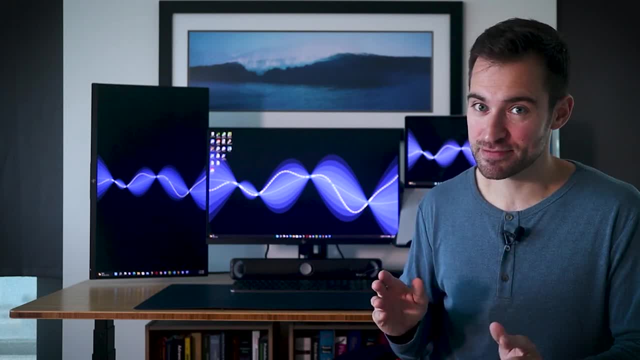 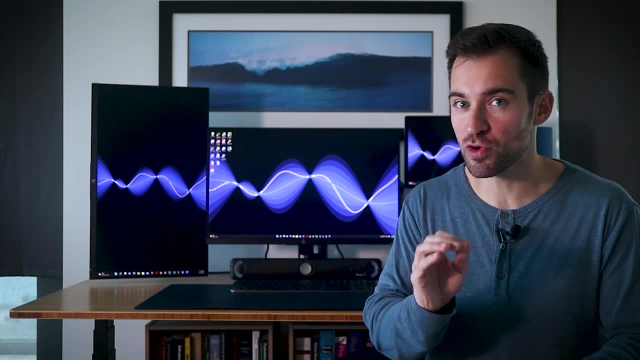 I saw my first clue of that at work And when I asked around, it appears this migration has already begun. As a starting point, let's use 2018, when Alexander Erpin, a Google robotics engineer, writes a piercing blog: Deep reinforcement learning. 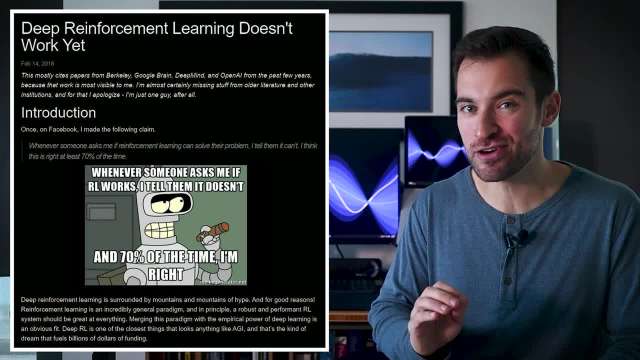 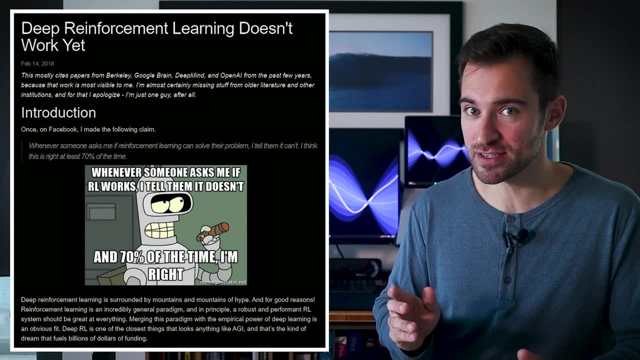 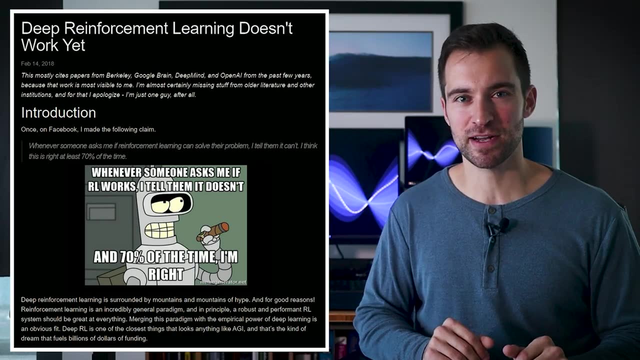 doesn't work yet. In it he explains that RL is just so damn data-hungry, unstable and requires so much tuning that it's really the best option for solving real-world problems. And because of this, you don't see it used that much. That was 2018.. So I emailed Alex for an updated perspective. 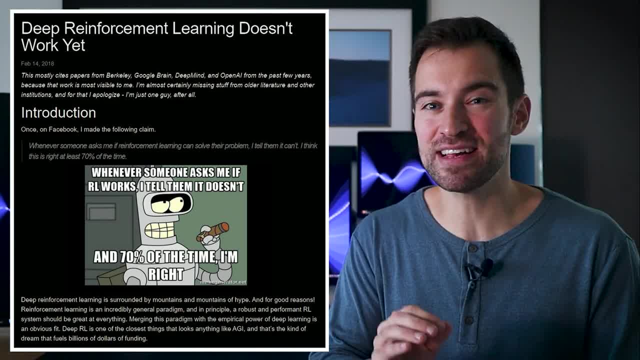 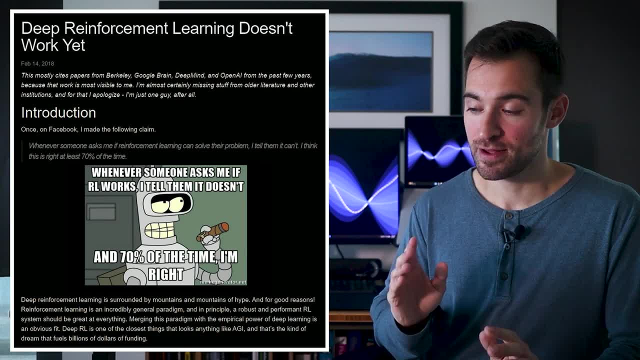 And he mentioned that since that post, he's seen evidence that RL is indeed being adopted in production at several large tech companies And that he's optimistic about the trend of RL. That said, he doesn't think that RL will be the same revolution that neural networks were. 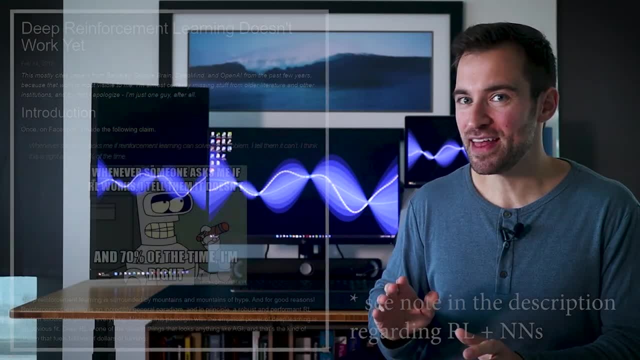 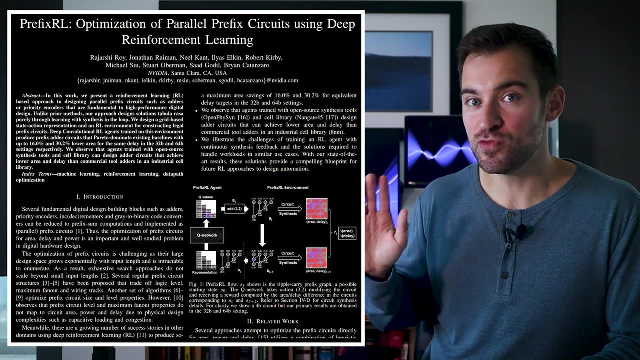 That's okay. Neural nets are quite a high bar, But beyond that, I found in the very recent past RL has been popping up as a useful tool For the real world. NVIDIA recently announced they've used Deep RL for designing more efficient. 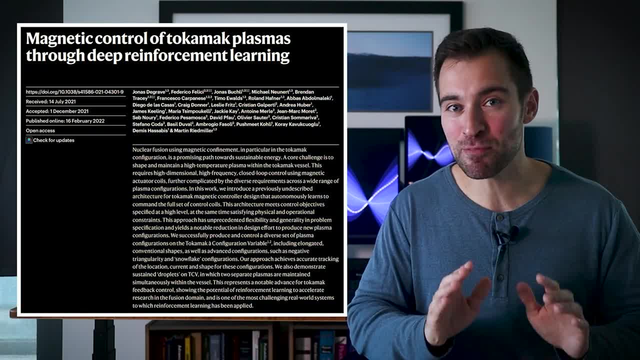 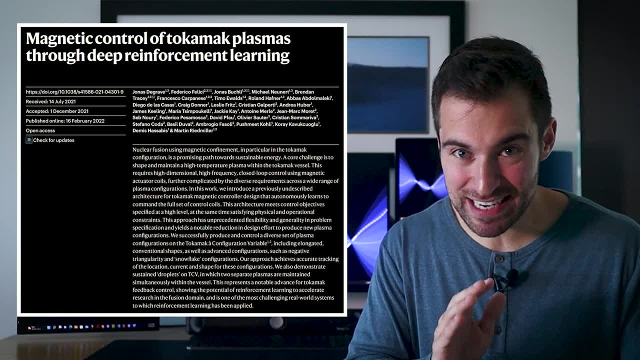 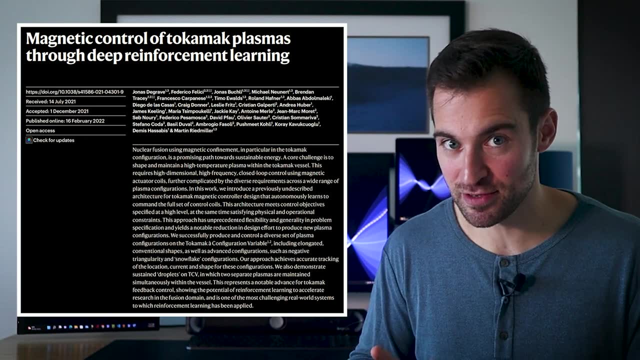 arithmetic circuits, DeepMind announced they can assist the operations of nuclear fusion by using Deep RL Specifically, their agent manipulates powerful magnets at millisecond timescales to contain nuclear plasma, which preserves the energy-producing reaction, Which is extremely cool, Not just useful. 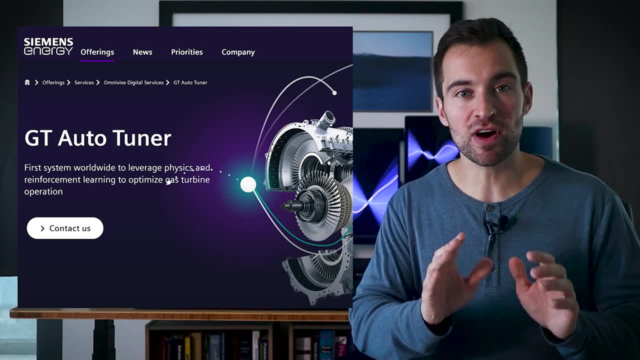 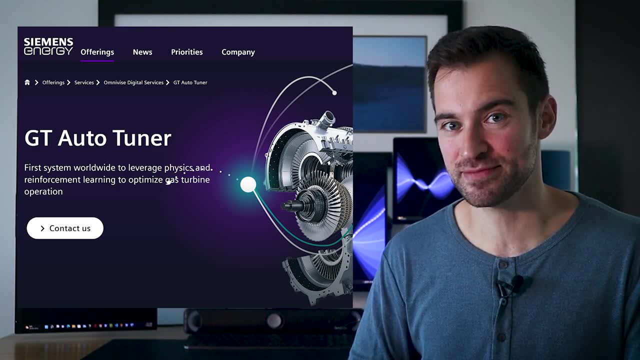 And speaking of energy, Siemens Energy uses RL to manage the energy efficiency and emissions of some gas turbines. This is something they've tested in the real world and used with their customers, And there are several other big examples which you can find in the description. 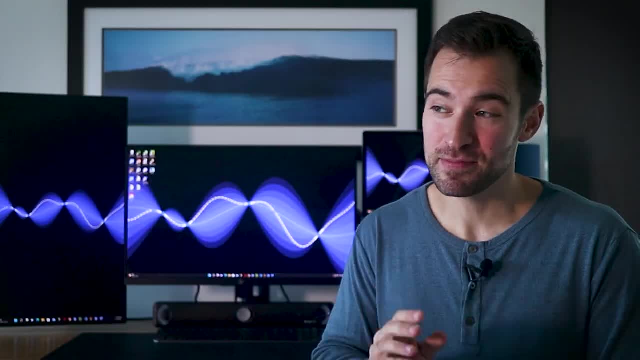 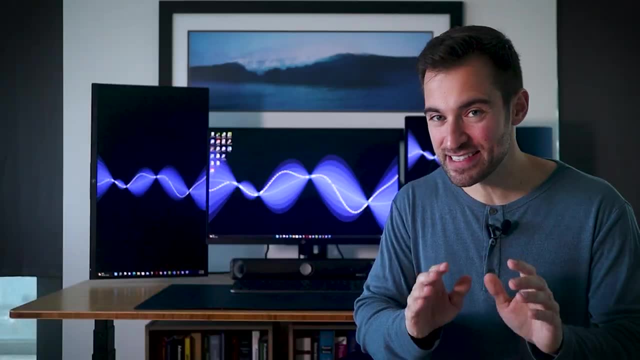 The point is, RL is certainly being used productively And there's a reasonable chance that this trend will continue, In which case knowledge of RL will be quite valuable, And that's where I can help To get these concepts into your head. 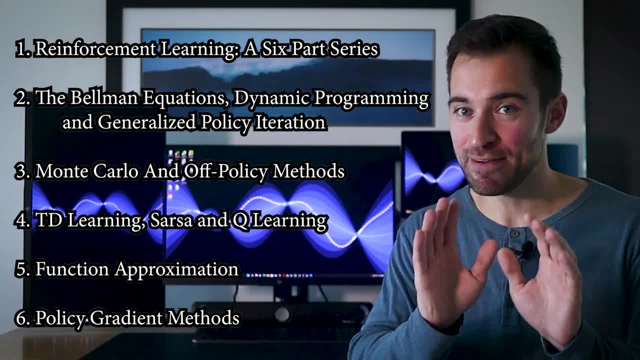 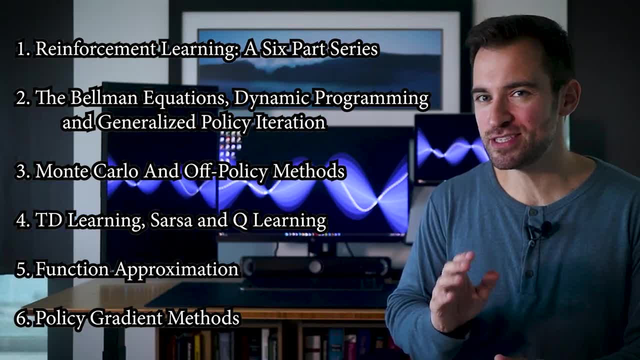 I'm announcing a six-part series on reinforcement learning. If you watch this series, focus hard and pause where you need to. you'll know the fundamentals. I can promise you that. Now, to put this into perspective, I'm going to talk a little bit more about RL. I'm going to talk 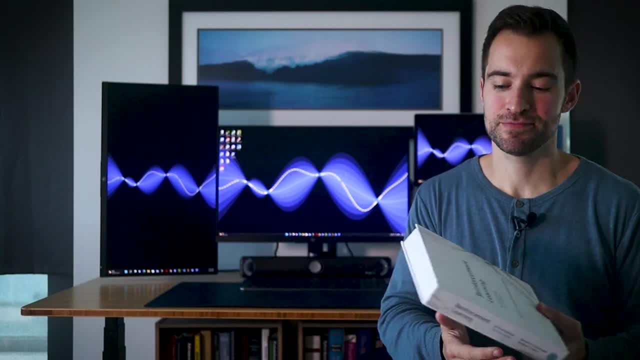 a little bit more about RL. I'm going to talk a little bit more about RL To put this series together. I've studied everyone's go-to textbook, Reinforcement Learning, An Introduction by Sun and Bardo. If you want a truly deep understanding, you should read this book. 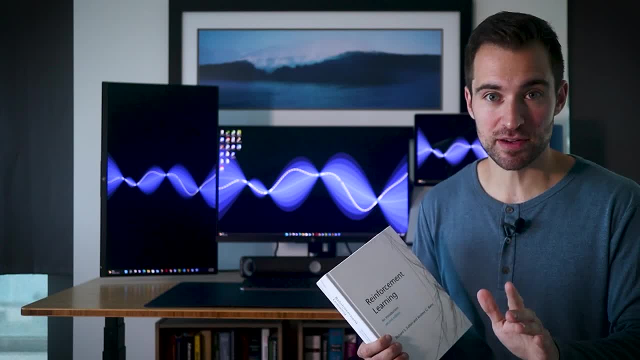 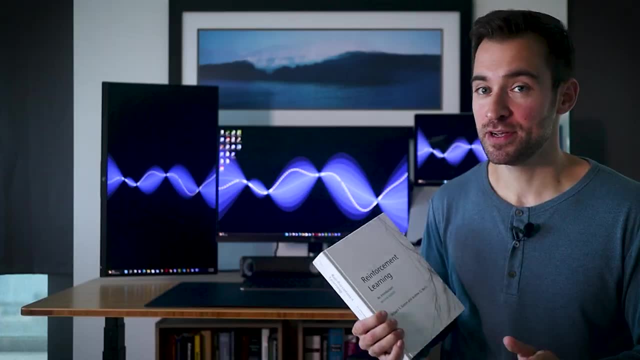 These videos will follow closely on core concepts. In particular, we'll cover much of part one and some of part two. All things considered, I think it's an exceptionally efficient way to learn. If you agree, there's only one thing left to do. 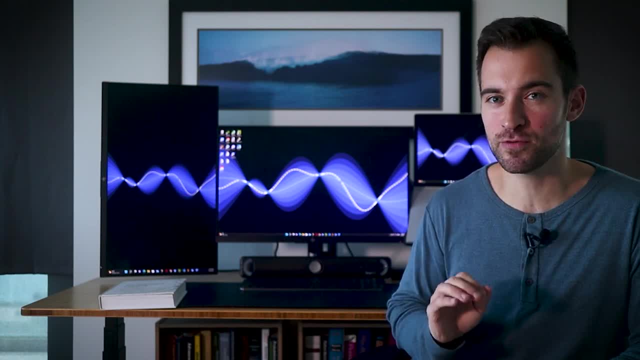 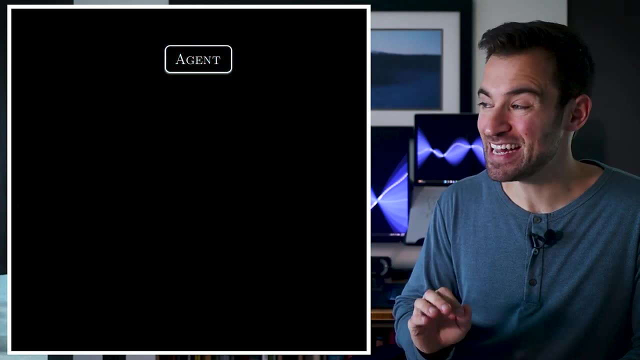 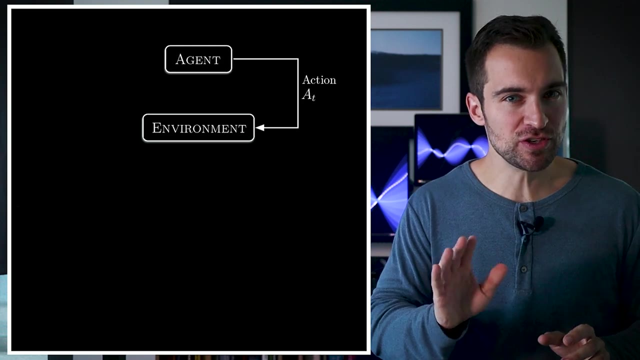 Get started. We begin with possibly the most important thing to know about reinforcement learning: The problem statement. It starts with the agent which represents that which learns and takes actions at each moment in time. t The action is then received by the environment, which uses that to produce a reward. 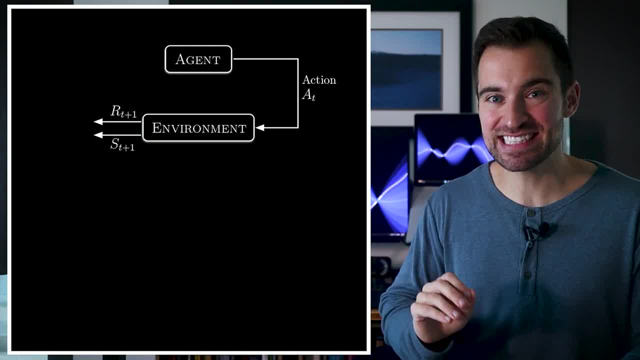 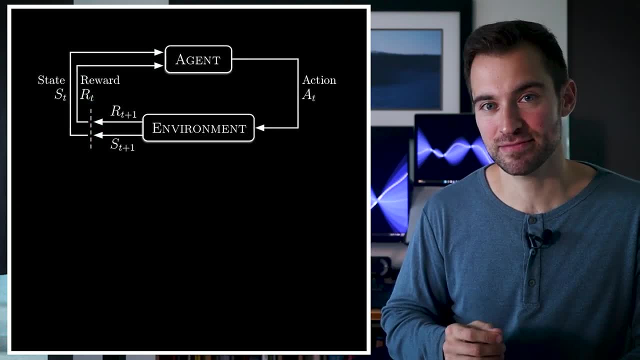 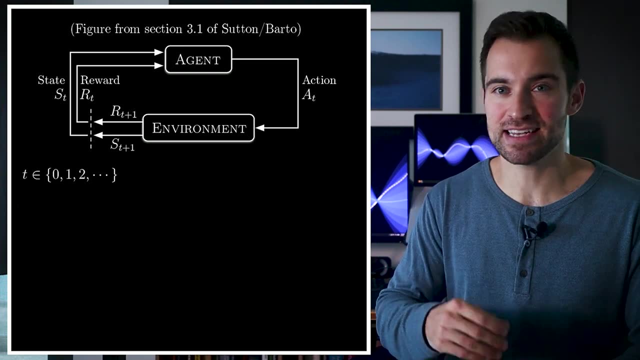 and a state at the next moment in time. This is then passed back to the agent for the next action to be decided. This line is to indicate that process repeats. So that's the general structure, but let's get more specific. First time is discrete, meaning it can be indexed as 0,, 1,, 2, up to whatever. 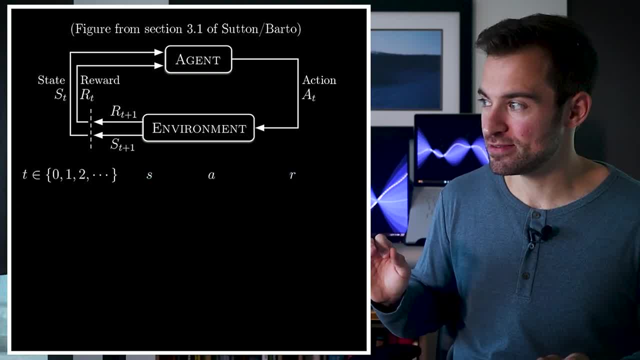 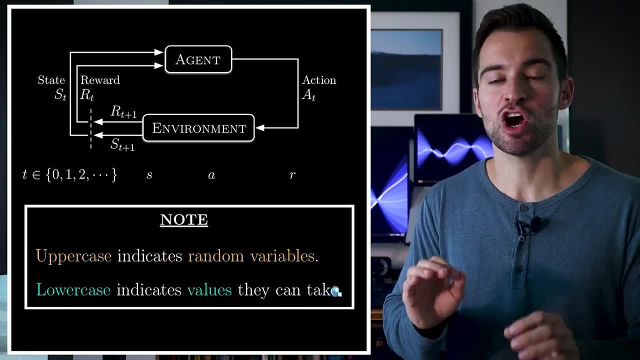 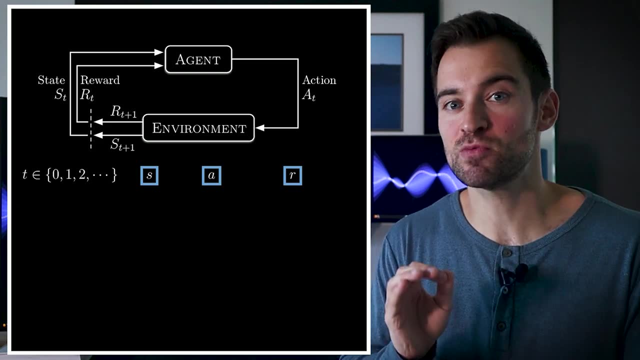 Next S, A and R. Now, before we discuss these, one note: Uppercase letters are random variables and lowercase letters are specific values those random variables may take. That means these lowercase letters represent values their respective random variables may take. 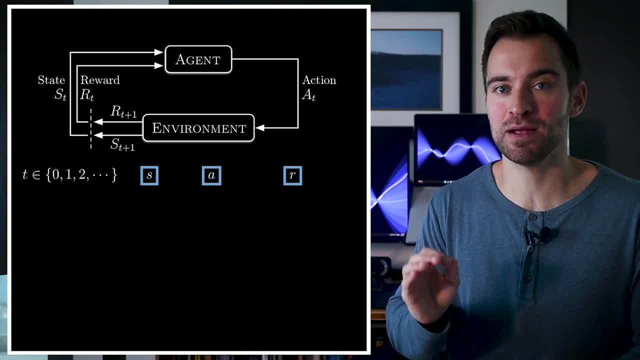 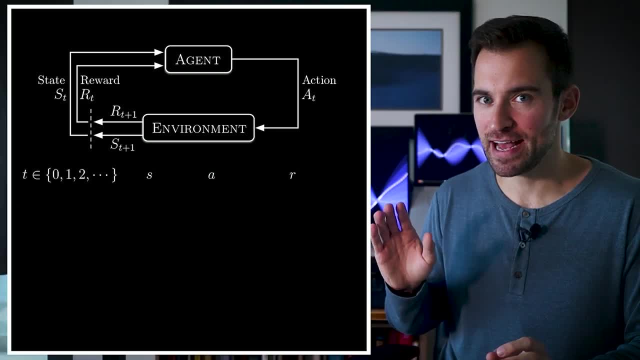 Those variables being the state, action and reward at some moment in time. With that, let's introduce notation to represent sets of possible values. First, S is from the set S written as S in calligraphy, which I'll call calS. 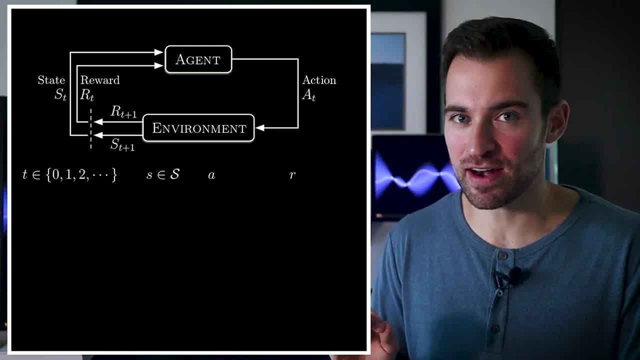 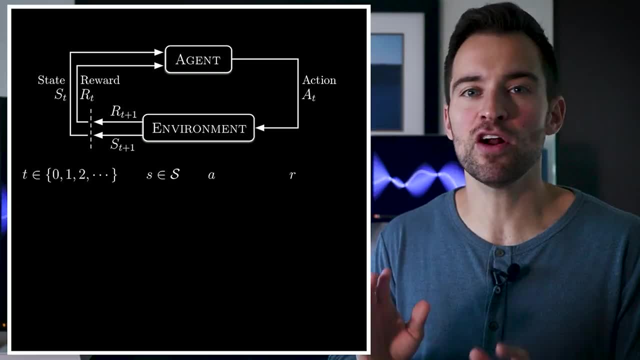 Now, calS is just a finite set of anything. Could be numbers or tuples, or animal names or colors, whatever It's there to indicate all possible states, whatever they may be. Next, A is in the set: calA. 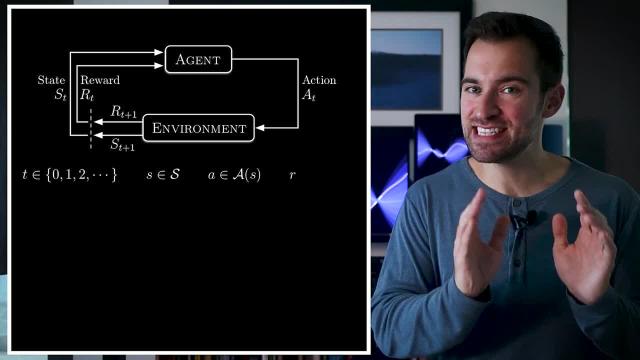 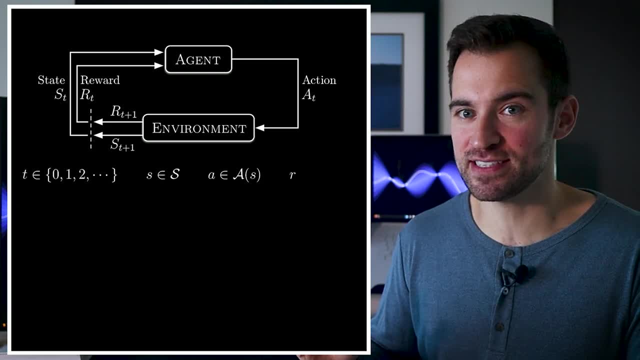 Next A is in the set calA. Next A is in the set calA. What this means is the set of actions the agent can take depends on which state the agent is in, And this is how we refer to that set. 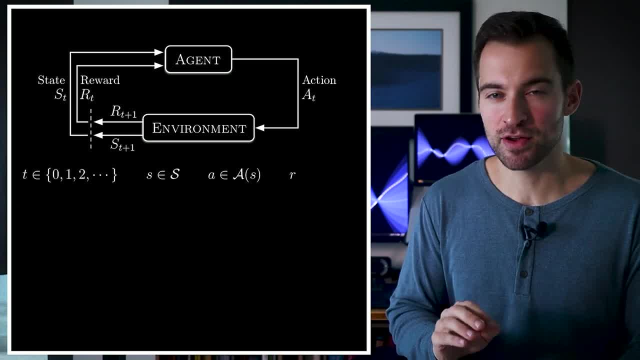 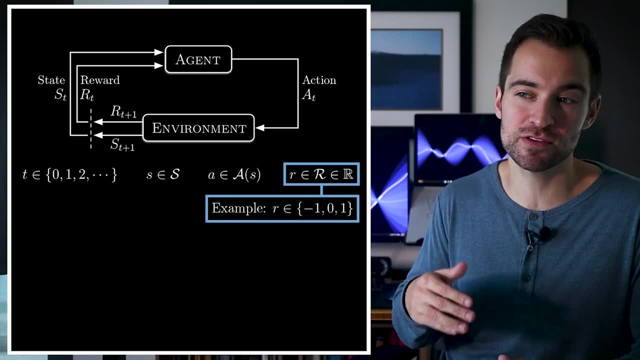 Got it. Finally, and this is where things get a little bit more restricted, R is in a finite subset from the real number line. As an example, it might only take the values minus 1,, 0, and 1.. Okay, the next part is quite important, so I'll need that focus. 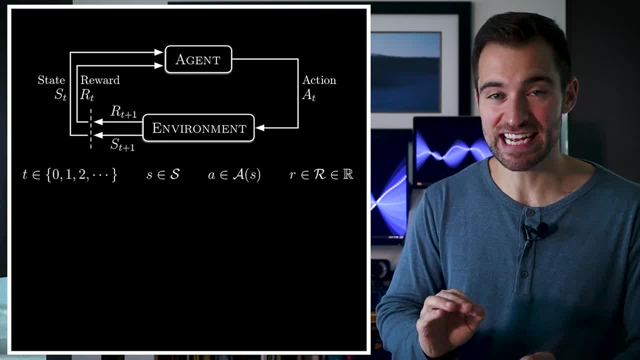 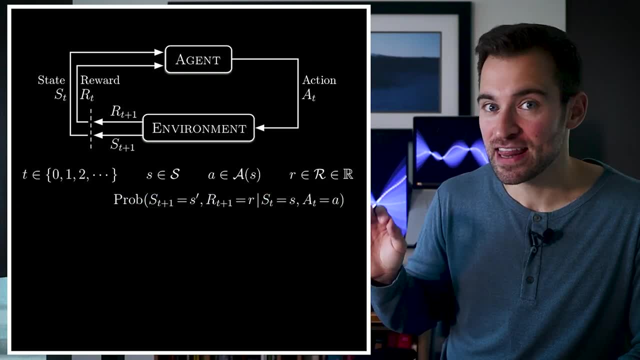 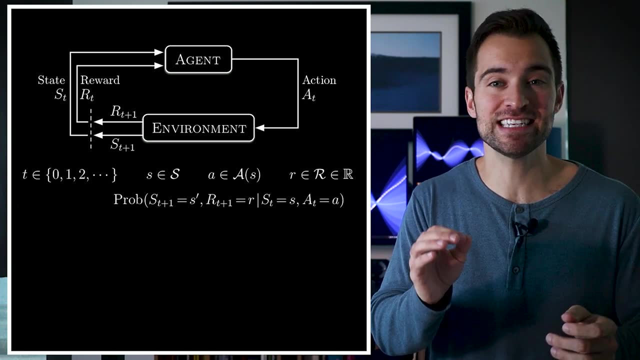 The dynamics of the agent-environment interaction is specified by a distribution function which we'll refer to with this. This function gives us the probability of the next state and reward being some values given the current state and some action to be taken. We'll write it like this for shorthand. 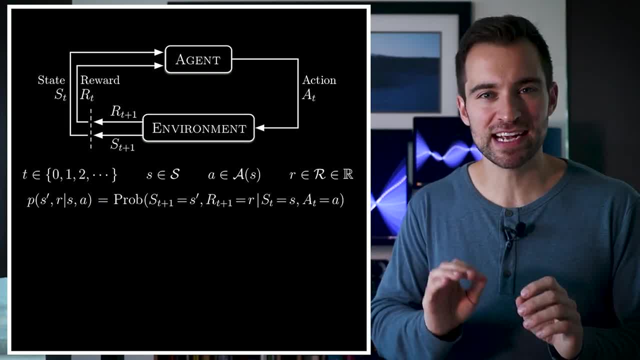 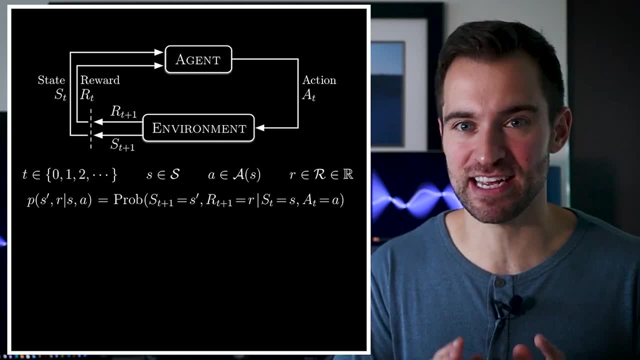 What's notable about this is that the probability of the next state and reward only depends on the current state and action. It does not depend on the history of states and actions, and that's a major simplification. This is called the Markov property, and it's, in fact, quite a strong assumption. 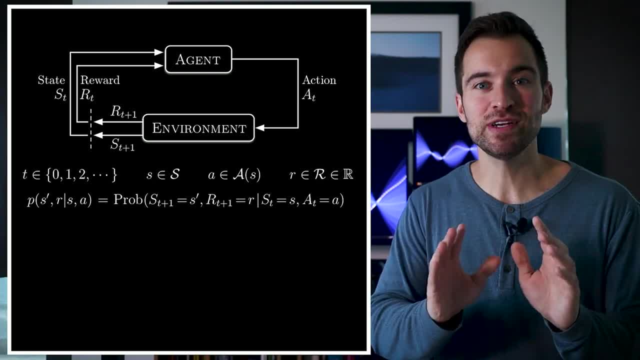 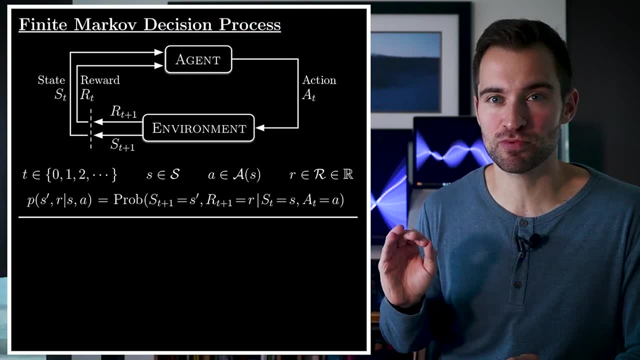 Now, taking a step back, we say the probability function and the finite sets of S, A and R define a Finite Markov Decision Process, or MDP for short. Got it? This is like the main object of RL, so make sure you digest it. 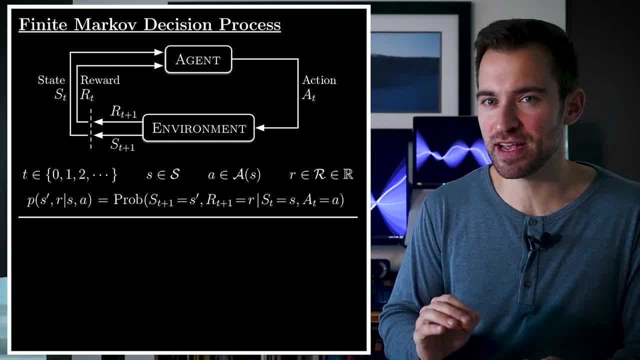 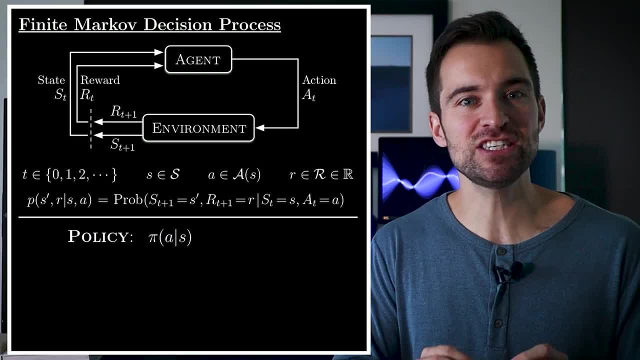 From here we can discuss the agent's behavior, which is given by the distribution function. Now let's take a look at the policy. It tells us the probability the agent will take each action when in a particular state. Think of it like a bar graph. 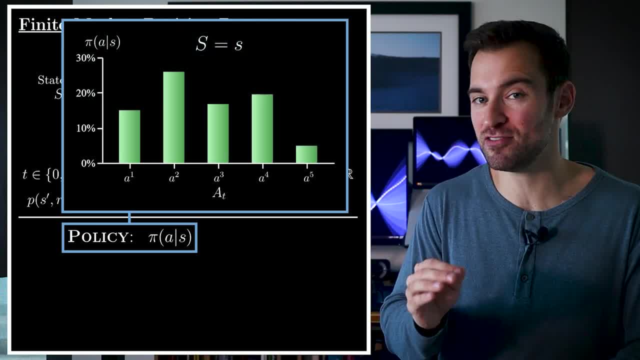 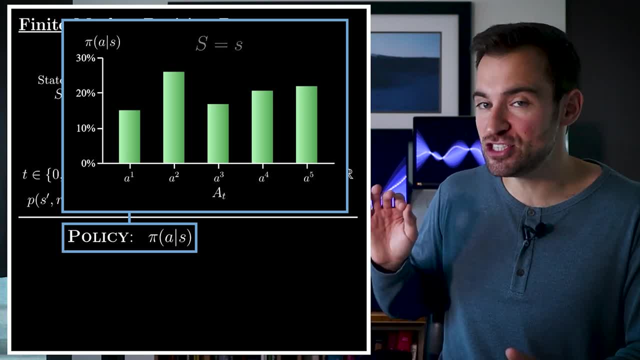 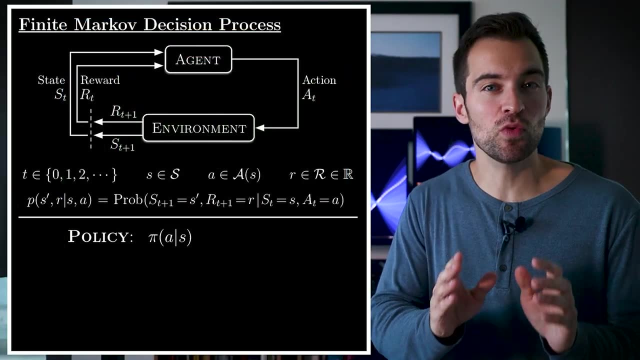 If the agent is in a particular state, the policy gives the probability of each action. The agent would then select an action by sampling randomly from this distribution. If the state changes, then so do the action probabilities Make sense. Also, if the policy involves no randomness, 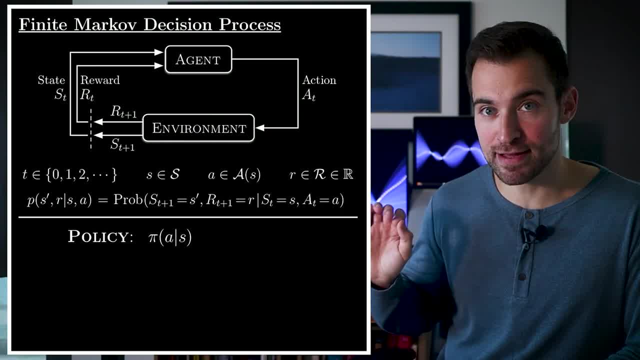 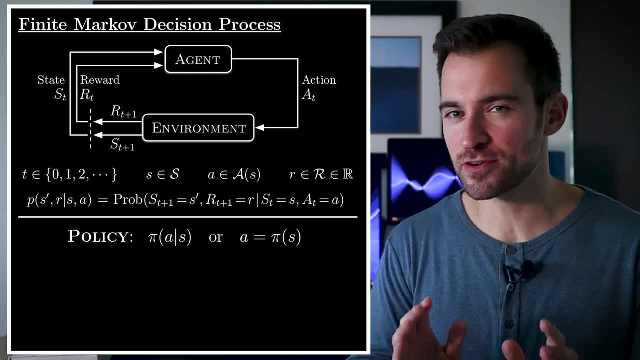 the action could be taken from each state. We write that like this. We say: the policy is Deterministic. Now this leads to an important question: What makes for good policy? Well, basically, we want a policy that will accumulate a lot of reward. 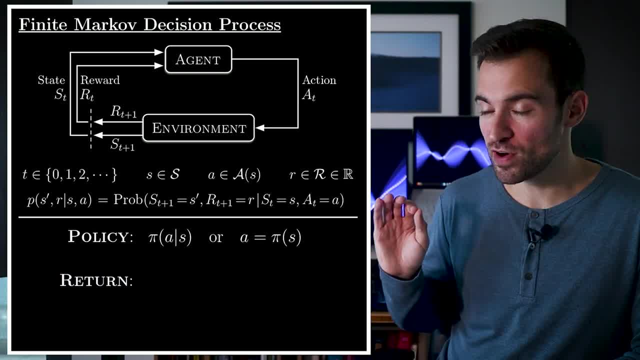 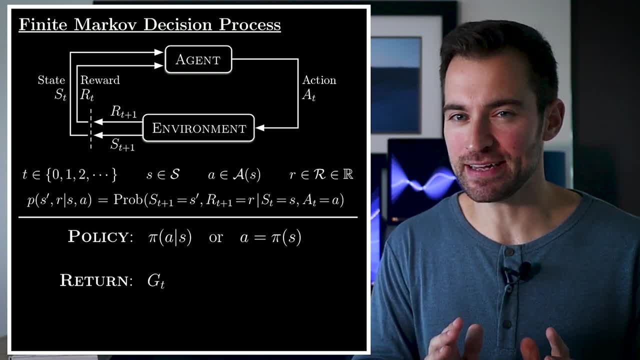 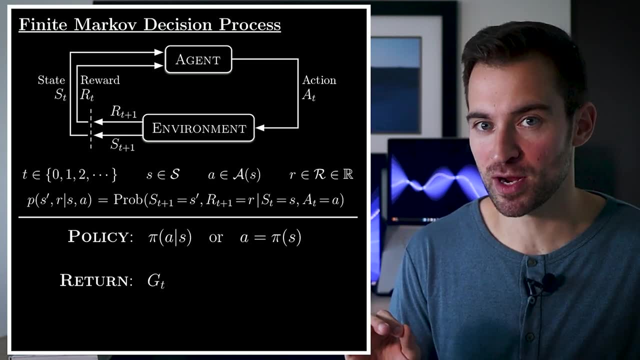 and we'll call that accumulation the return. We write the return as GT and it's essentially a sum over future rewards, Though not exactly Because we may want to give sooner rewards more weight than those further in the future. we will also add a discounting parameter. 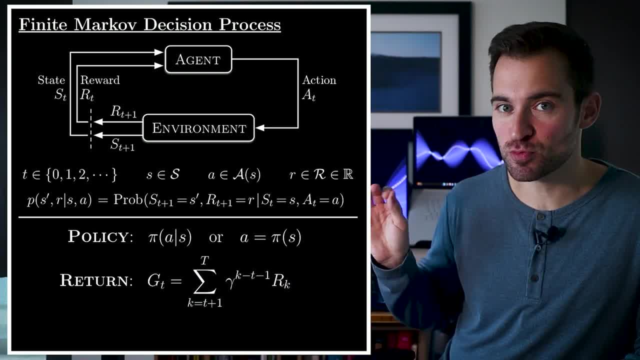 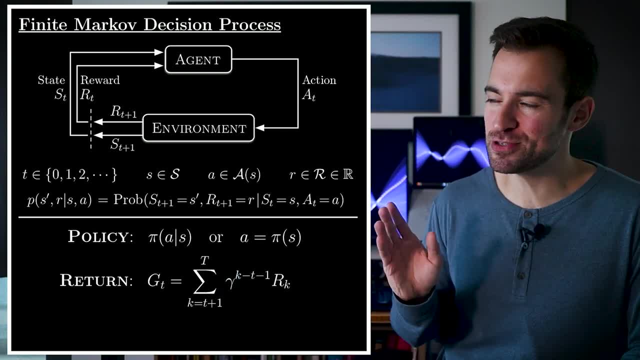 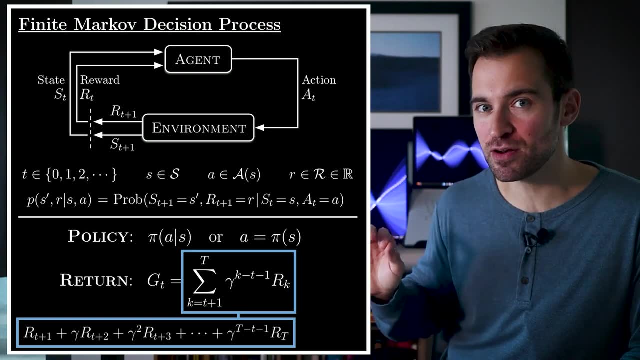 Specifically we say: GT is this expression where gamma is our discount parameter between zero and one. It may help to expand this out a bit Here. you can see the return is just a sum over future rewards discounted by gamma, according to how many steps they are. 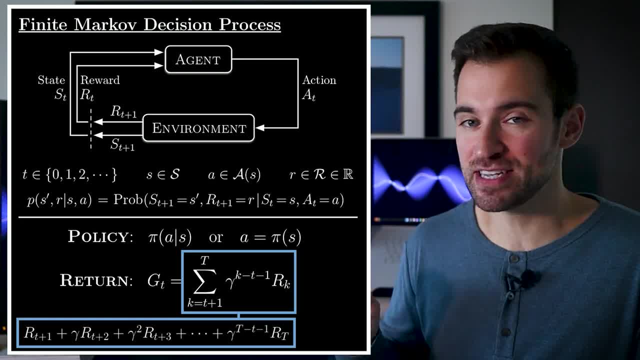 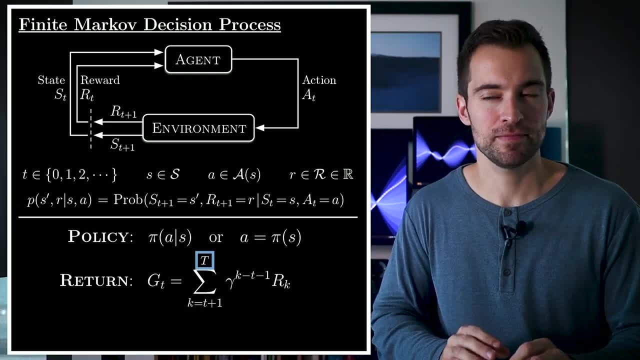 from the current time. Hopefully it's clear: the closer gamma is to zero, the more you weigh near-term rewards. One note here: I've introduced the final time T In the book. you may see infinity here. The reason for that is the book considers two cases. 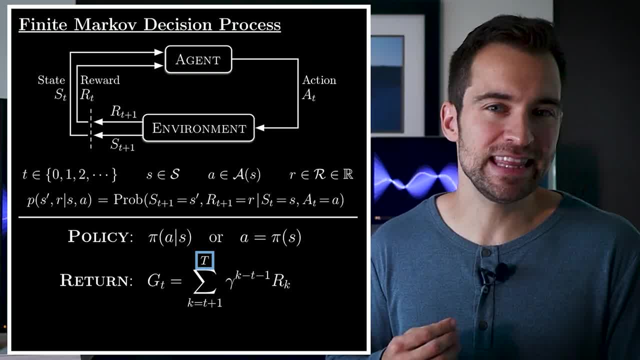 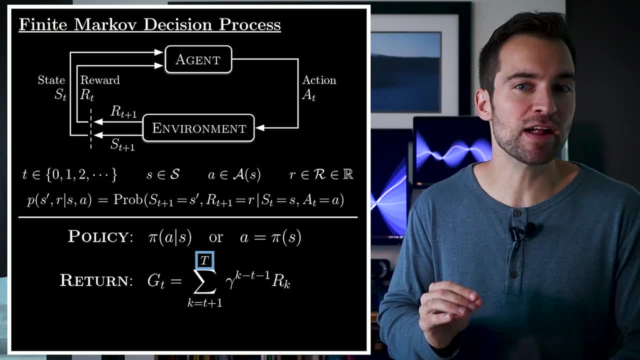 called the continuing case and the episodic case. In these videos I'll for the most part only discuss the episodic case. In the episodic case, running the policy through the MDP comes to a definitive end, marked by entering a special state. 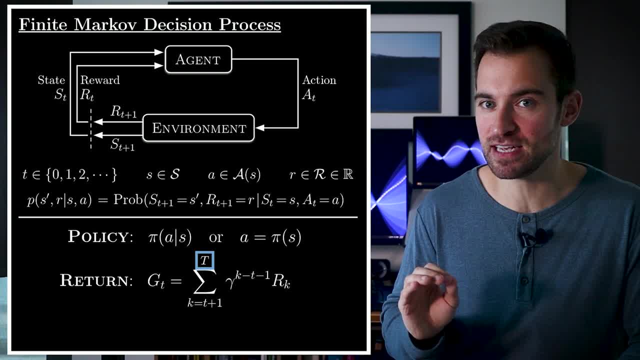 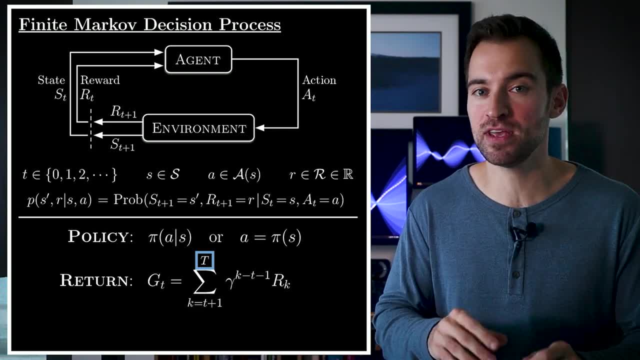 called a terminal state And that's a time capital T And that marks the end of what we'll call an episode. At that point we can rerun things through the MDP to produce another episode Regarding notation if we include the terminal state. 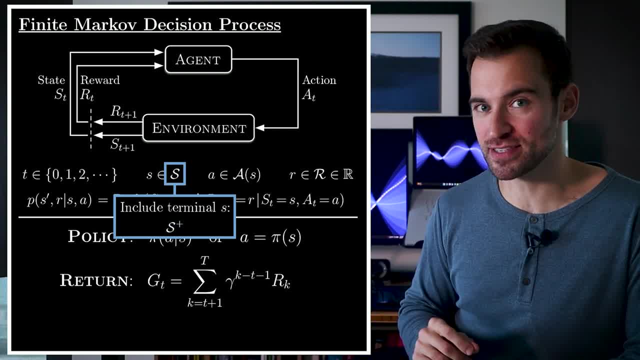 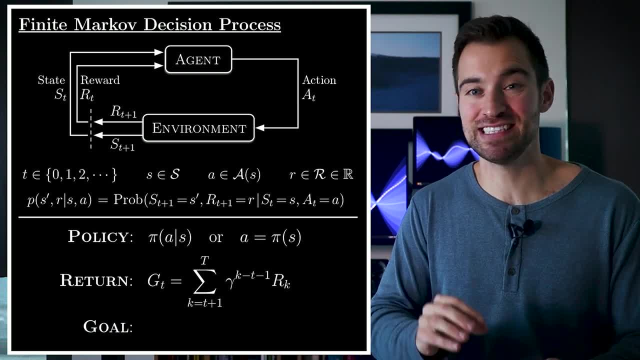 in the set of states, we refer to that set as CalS plus. With that we can be more precise about the goal. The goal is to select a policy that will maximize the expected return. That is, if you run a policy through the MDP with many 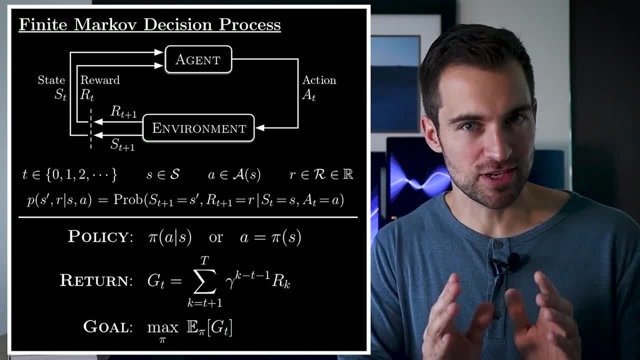 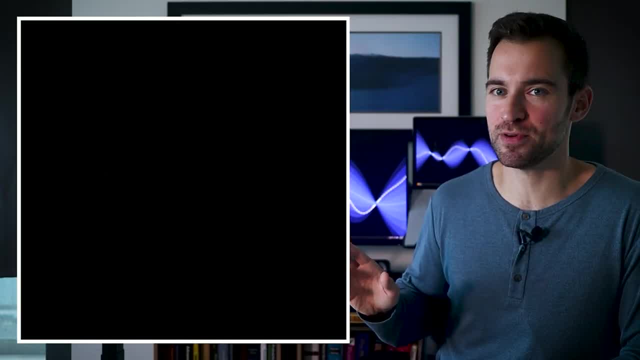 episodes. on average, you'll get a certain return, So pick the policy that has the highest average return. That's the name of the game. OK, let's visualize this with an example. We'll start by listing out the possible states as different shades of red. 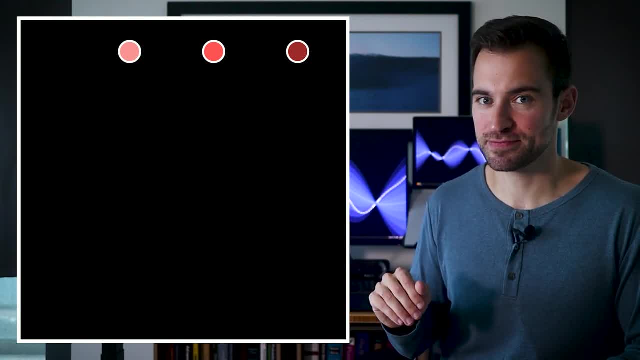 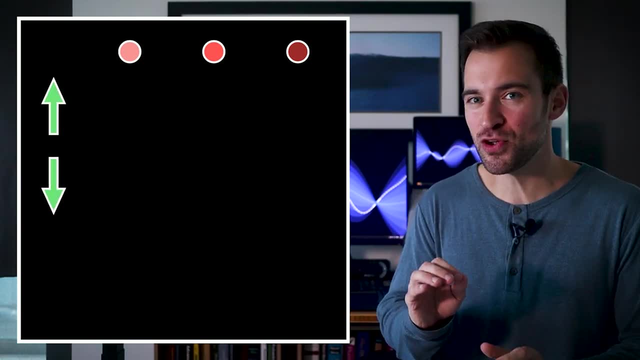 States can be anything. So just to demonstrate, I'm going with colors. Now, in each state the agent could take one of two actions: up or down. Now I'm going to show you how we can think of the MDP probability. 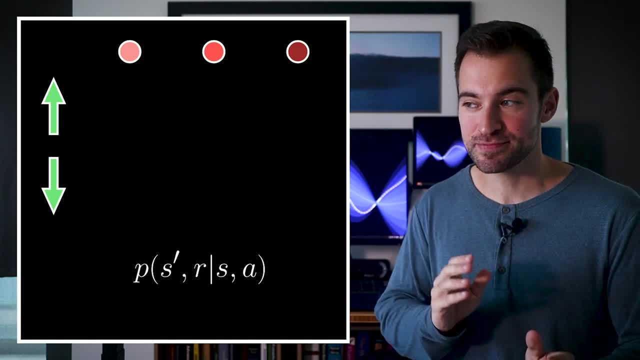 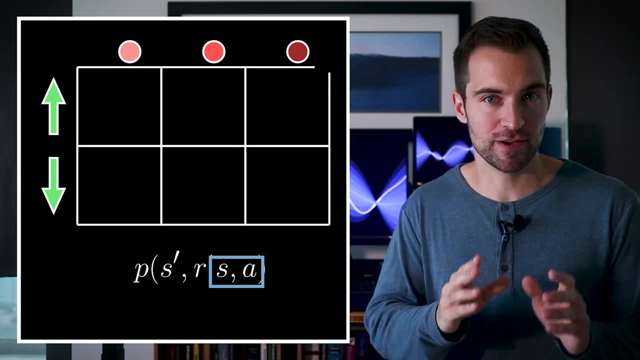 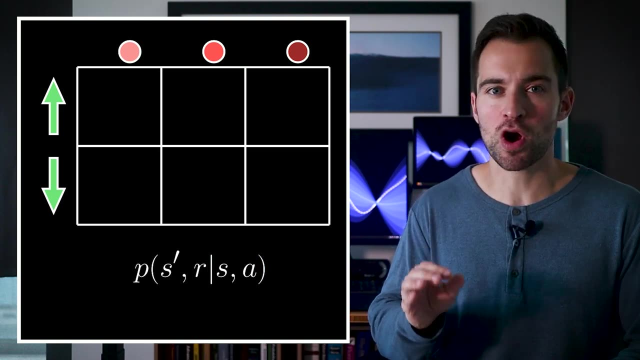 function. The colors and arrows, states and actions are my way of laying out the conditional part. That is, for each combination of state and action we will have a distribution over the next state and reward. Let's say the possible rewards are minus 1,, 0, and 1.. 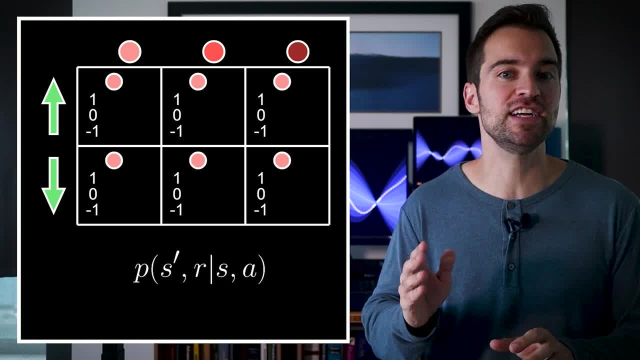 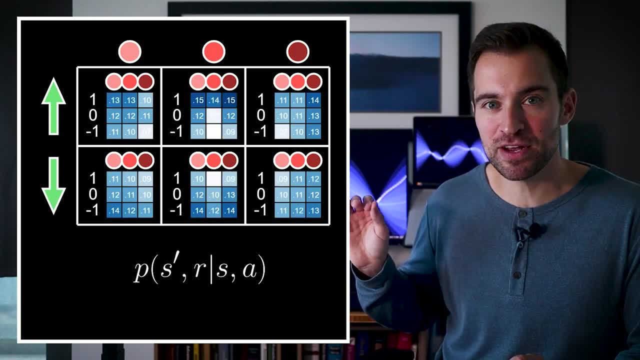 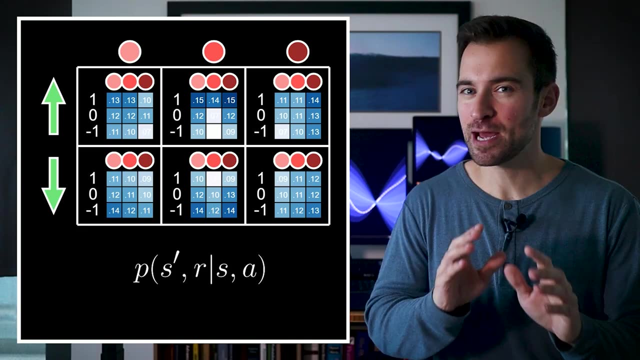 Also, the possible next states are, as required, the shades of red. Now we can picture these distributions as heat maps. Each heat map here gives you the probabilities of getting a certain pair of next state and reward, given the current state and action. 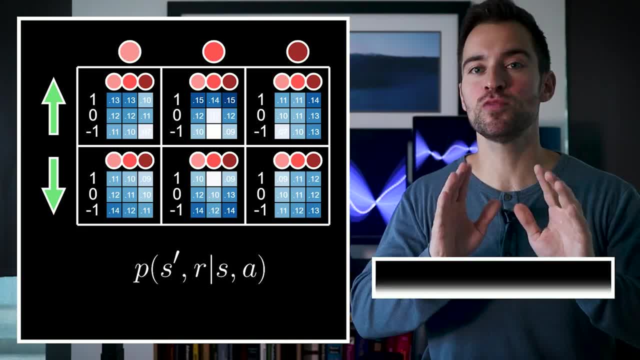 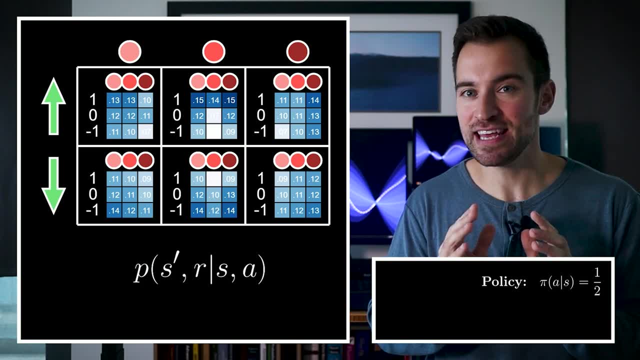 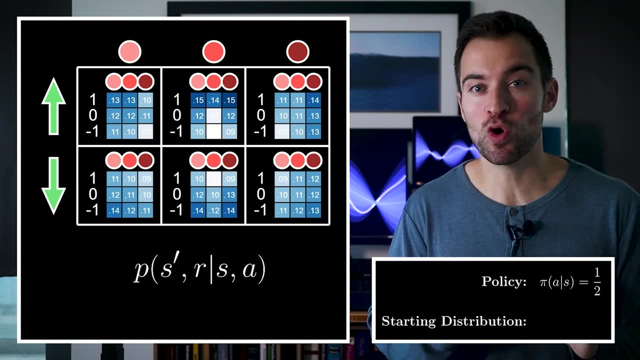 Now, before we can simulate an episode, we need to specify two more things. The first is our policy, which, I'll say, gives equal probabilities to the actions in all states. The second is something we haven't mentioned: We need a starting distribution over the first state. 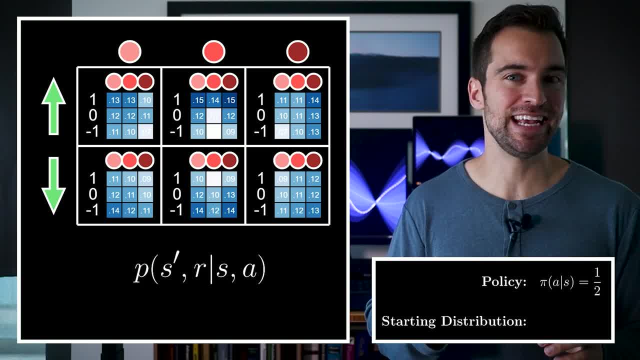 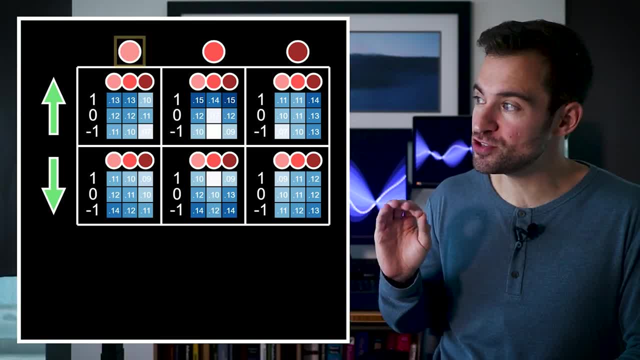 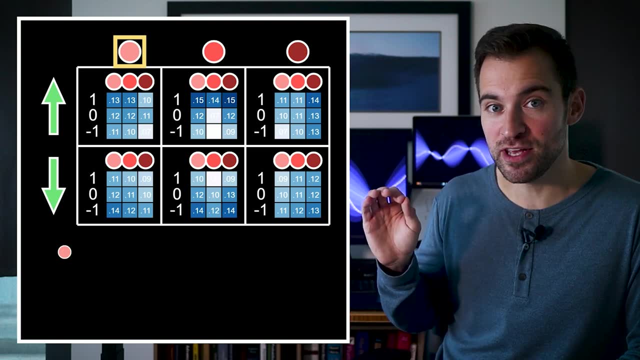 since there is no preceding state in action. In this case we'll say each state is equally likely. Finally, we can simulate an episode. First, we'll use the starting distribution over states to sample the first state of the episode. From here we use our policy distribution. 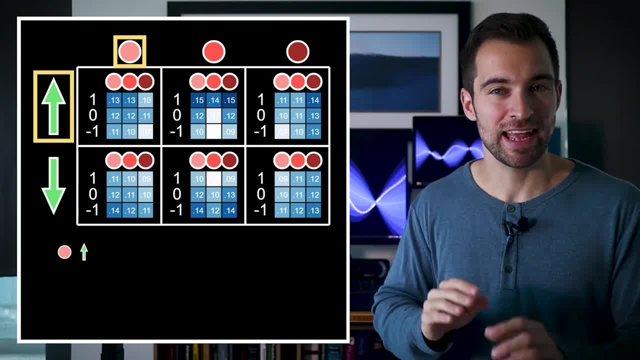 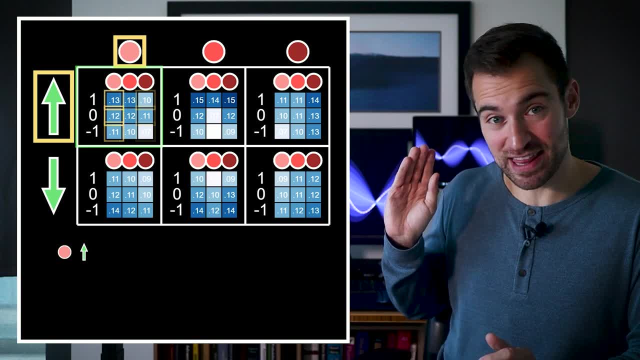 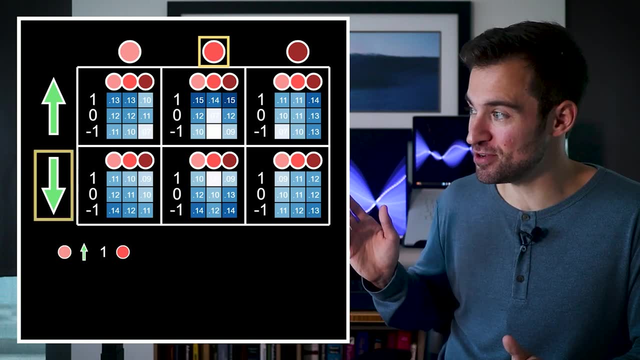 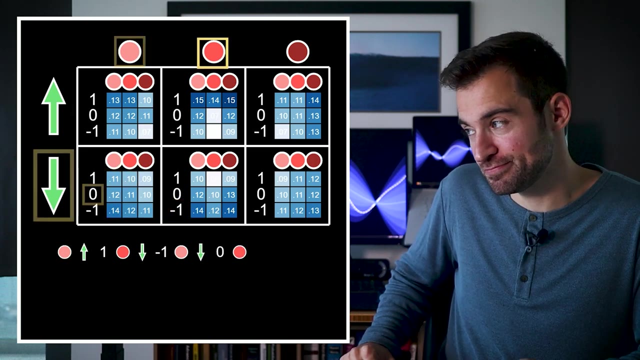 to sample a particular action. These two tell us which distribution over next state and reward applies. Sampling that gives us a policy distribution, It gives us a pair of reward and next state, And this process continues. You get it Now. I did leave one thing out of this example. 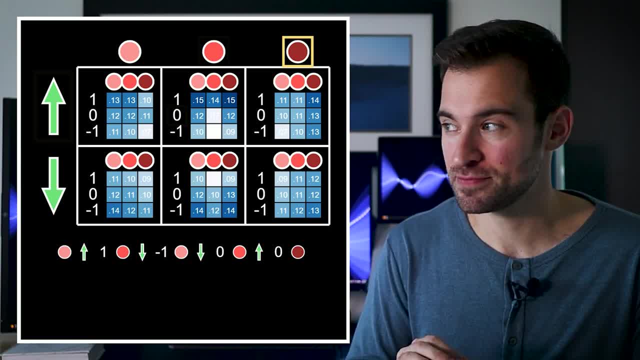 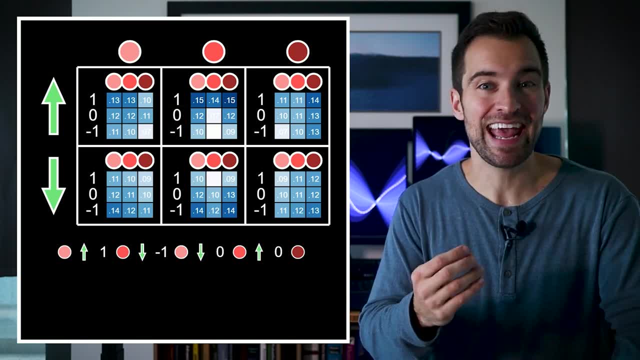 the terminal states states that mark the end of an episode. As illustrated, this process would continue indefinitely. Instead, there should be a terminal state which, if sampled, ends the episode. I'm comfortable leaving that to your imagination. Following termination: the process. 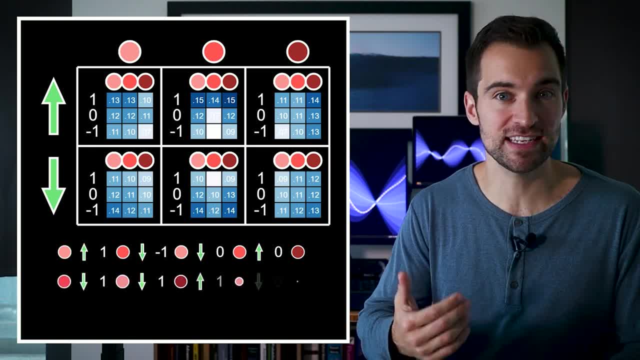 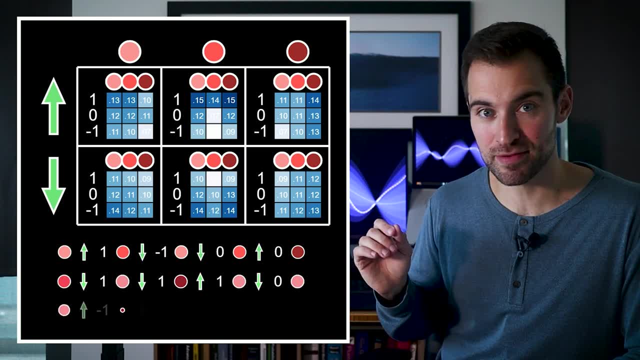 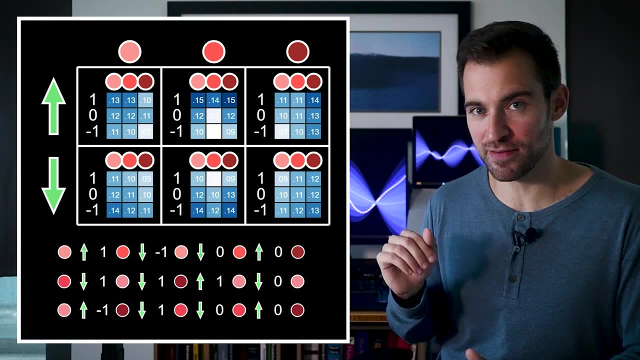 repeats for another episode and we'd get another sequence of states, actions and rewards. We'll call one such sequence a trajectory, and it's easy to get another. Ultimately, our data will be made up of many of these, though, you should note, most often they won't all. 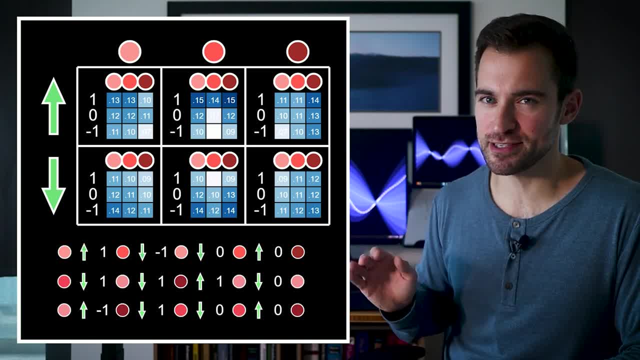 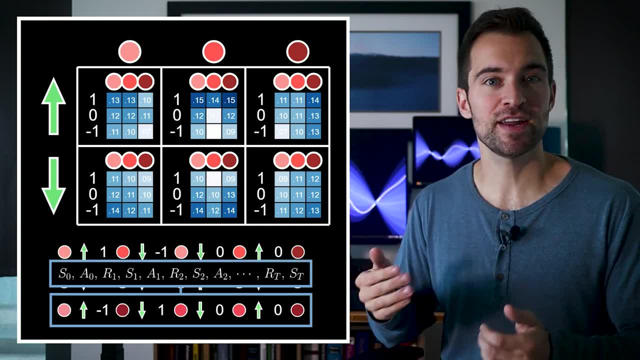 have the same length like this. Also, writing trajectories like this is a burden, so you may see it referred to as random variables like this Also, later you'll see me refer to their values like this, where m is to indicate the mth episode. 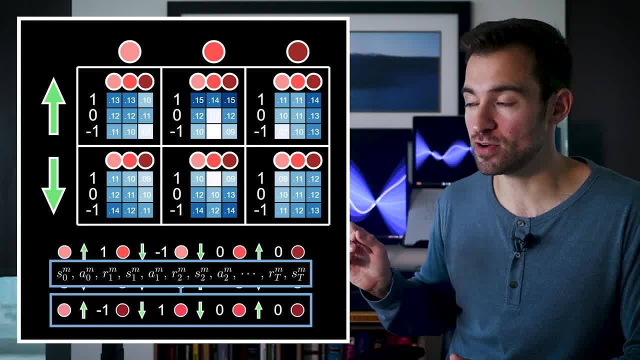 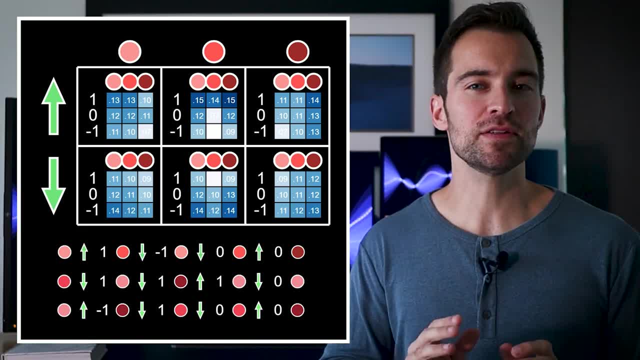 Since this refers specifically to the third episode, m would be three. As a final note, as I've shown, the policy is fixed the whole time. In reality, we're likely to learn the policy over time, so the policy changes between trajectories. 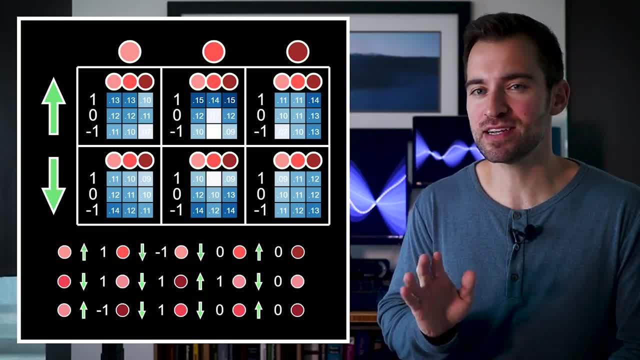 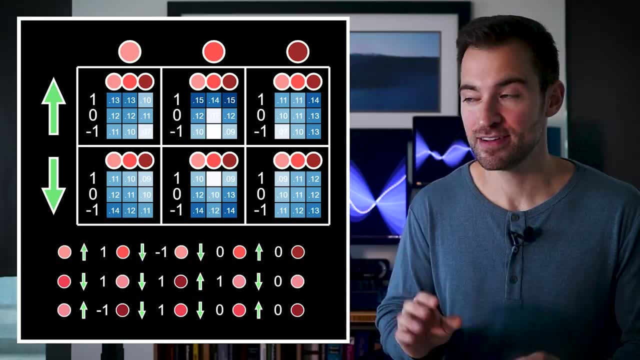 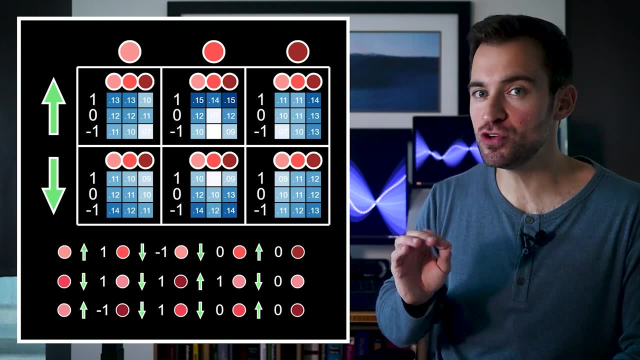 and sometimes within trajectories. This also highlights the complexity of reinforcement learning, Your answer to the problem. The policy also determines how data is collected. That's very different from supervised learning. Now, hopefully, from this position, the goal seems more clear. We want to choose our policy such that the rewards 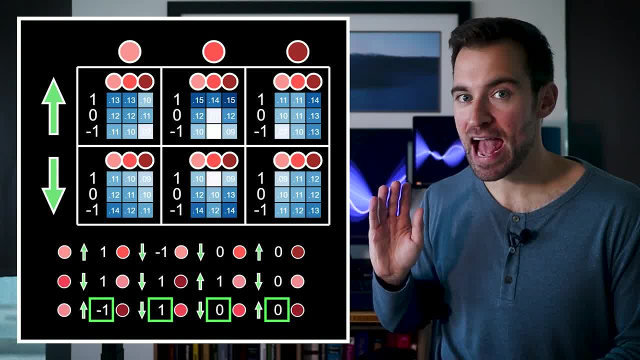 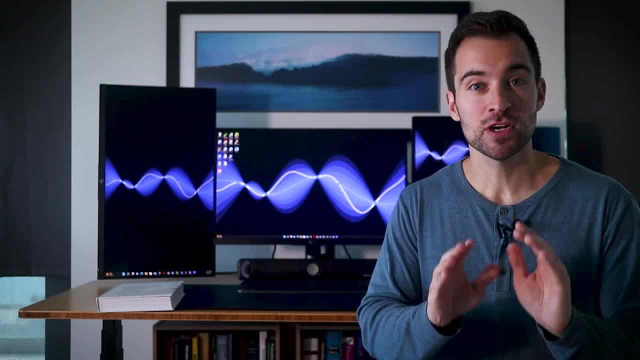 when discounted, add up to something high, averaged over many trajectories. Again, that's the game At this point. I've thrown a lot at you, so take a two, maybe three-second break. Great, Now we're ready to ask: how do we determine a policy that'll? 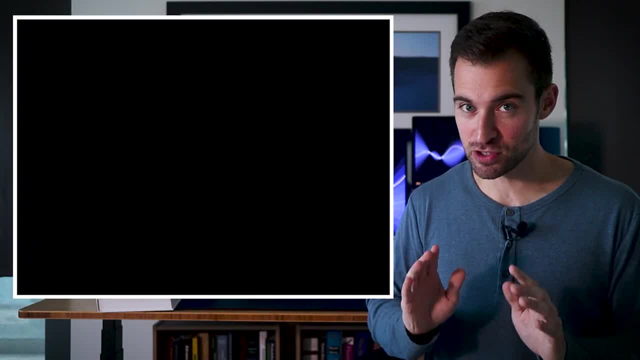 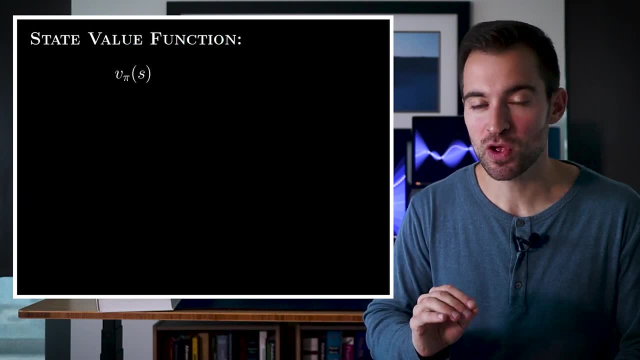 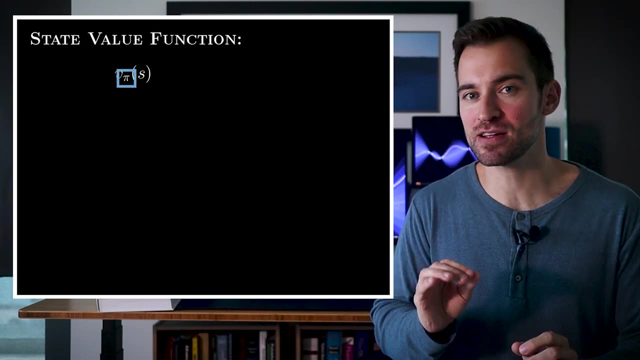 accumulate a lot of reward. Well, that's a huge question, But to start we can introduce two extremely important functions. The first is the state value function, which accepts a state and returns a number. The subscript indicates this function depends on the policy pi. 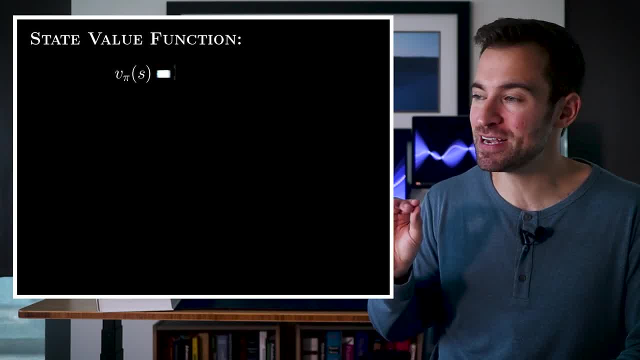 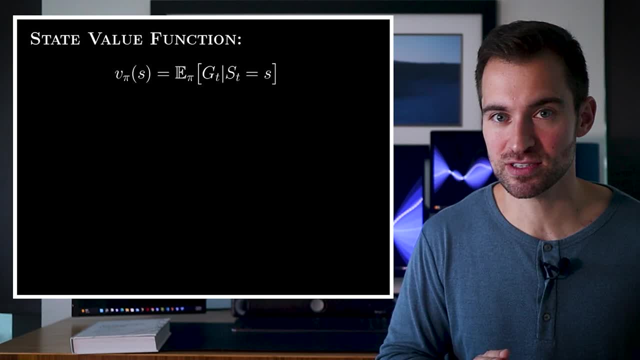 OK, now this function is defined as the expectation of the return, given the agent is at state s and uses the policy pi to determine its future actions. If we recall our goal from before, we see how closely related this function is to that goal. 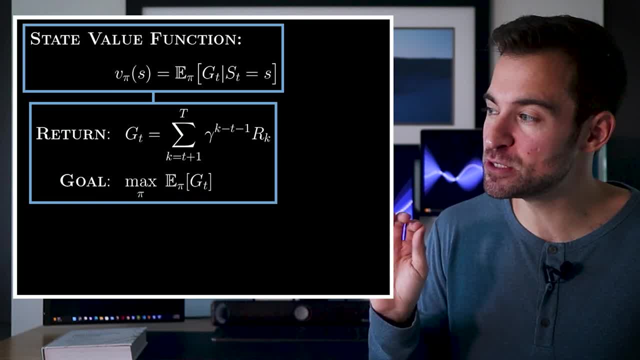 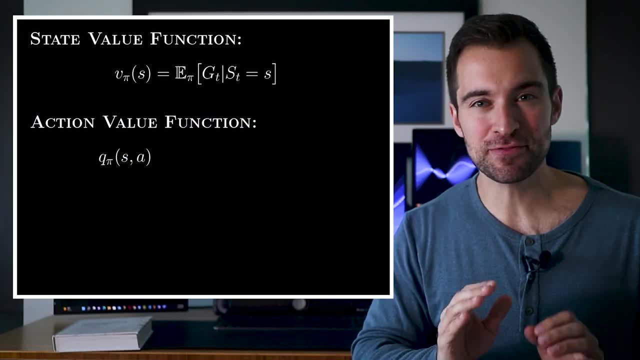 The value function is what we are trying to optimize, except it's broken down by state. And in a similar vein, we'll break it down even further with the action value function. It's defined in the exact same way, except we also condition on the action. 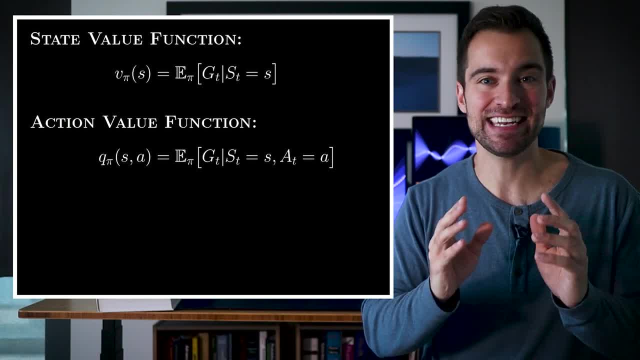 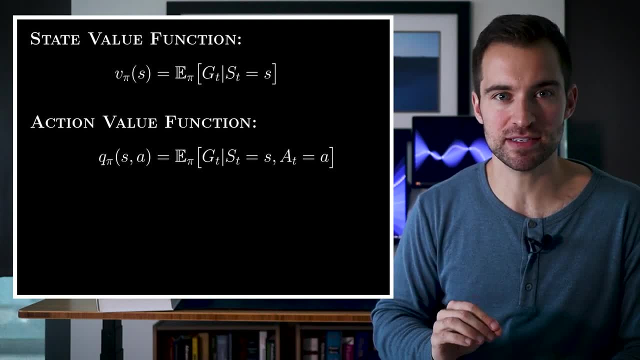 It's the expected return, given the agent is at state s and takes action a and then follows pi after that. As we'll see, these functions are very similar. These functions are crucial for finding optimal policies, But, as we'll also see, knowing them exactly. 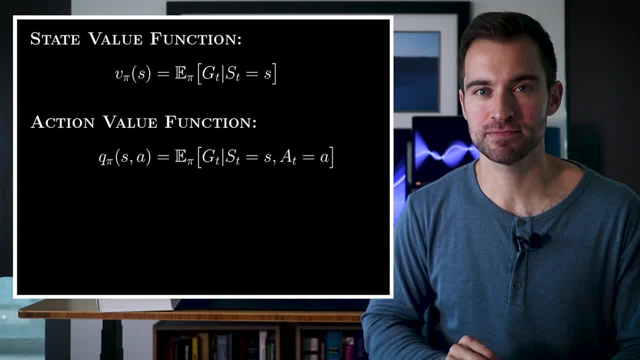 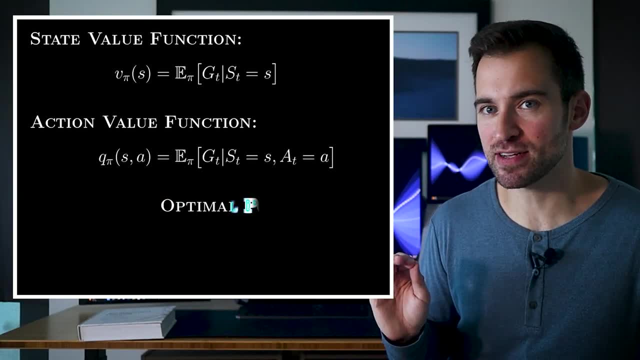 will typically be impossible, And we'll have to settle for estimates. Let's ignore that difficulty for now and instead ask what makes these useful? Well, the goal is to find an optimal policy, which we refer to as pi star. Now it turns out, they can be defined via their value. 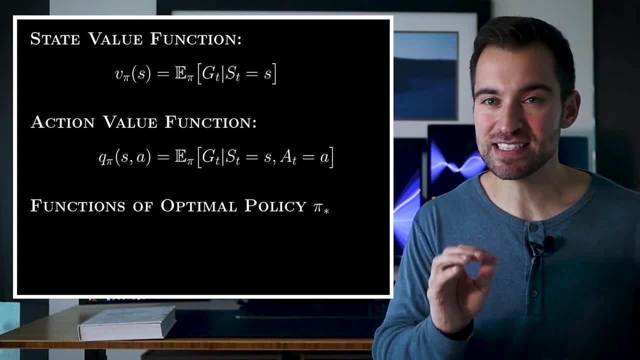 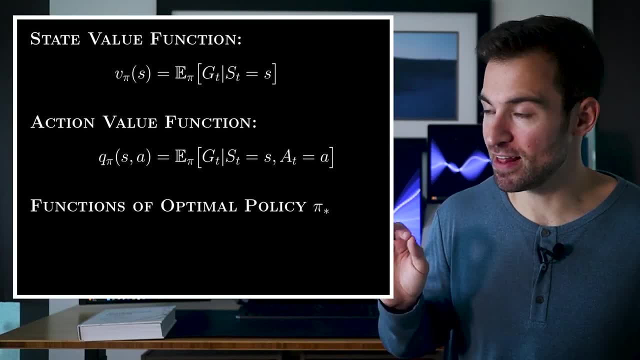 functions. That is, we say a policy is optimal if it achieves the highest possible expected return for all states. We can express that like this: If you're observant, you may wonder if such a policy even exists. The answer is yes. 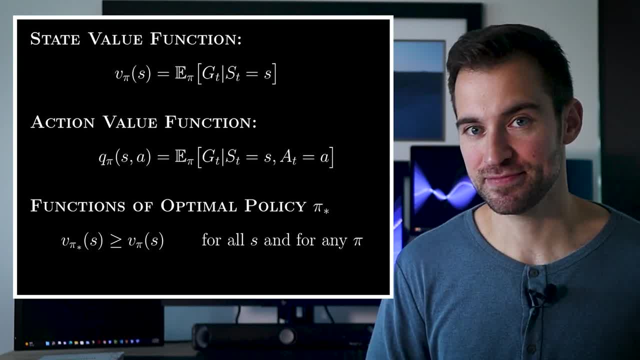 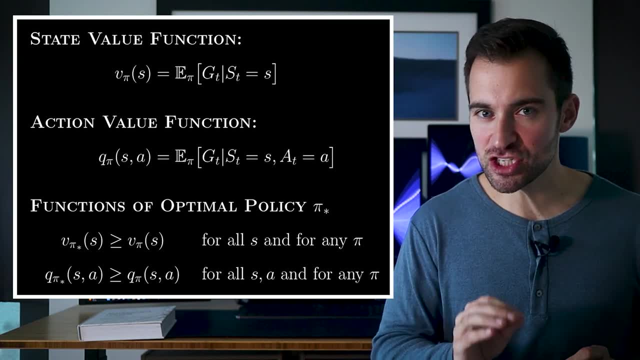 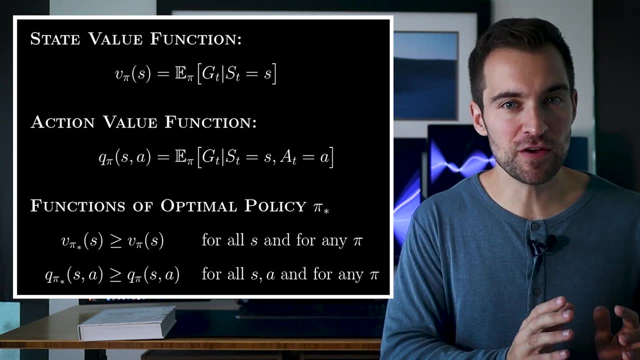 It's a proven fact that there is always at least one optimal policy, And similarly, the exact same idea holds for action value functions as well. Again, the only thing that changes is we're conditioning on state action pairs instead of states, As we'll see in the next video. state value functions and action. 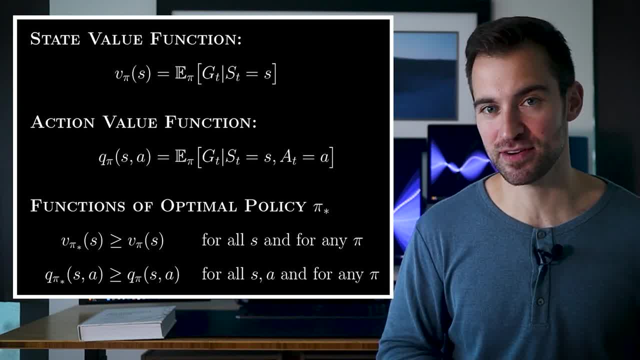 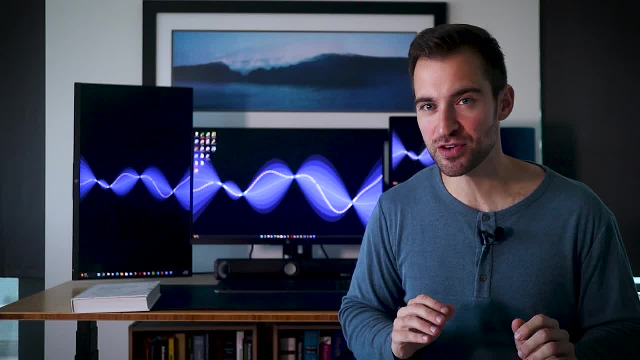 value functions of the same policy are tightly related to each other. Also, sometimes we'll abbreviate notation like this to refer to optimal policies. Now, to demonstrate how these are useful, let's consider an example. Let's say the agent is faced with a maze. 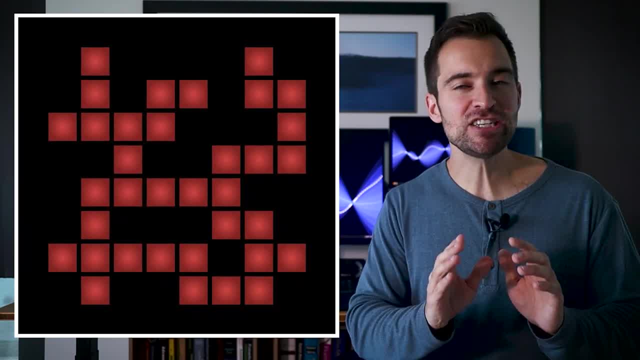 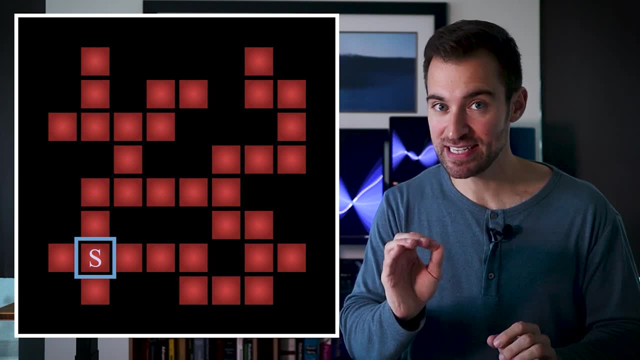 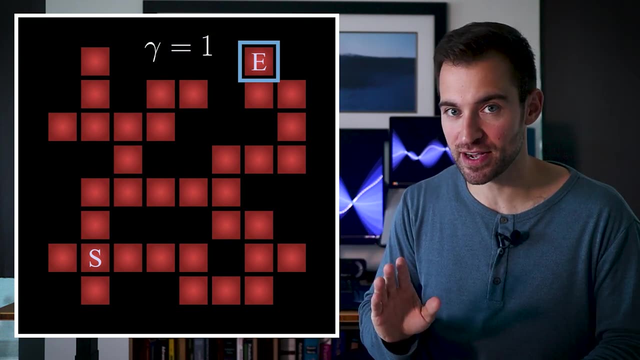 Each cell here represents a state. The agent begins each episode here and each step taken incurs a negative reward of minus 1 until the end state is reached and the episode ends OK And gamma is 1.. So no discounting. 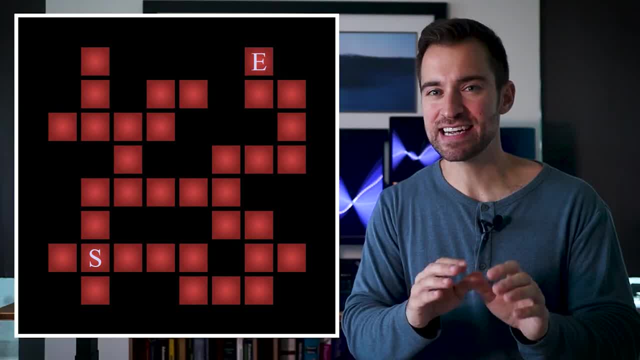 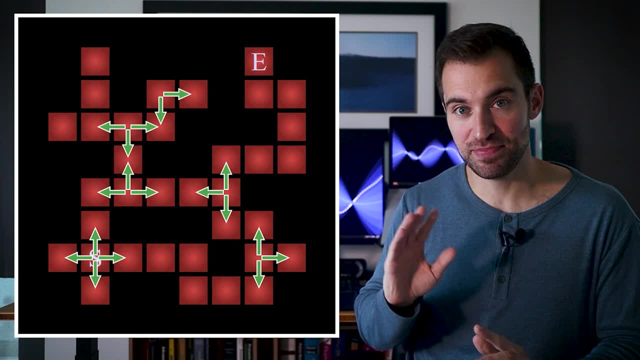 Clearly, the goal is to get to the end state as fast as possible. Next, the agent's available actions are to select a direction towards an available next state. Also, the environment is deterministic. The action without randomness fully determines the next state. 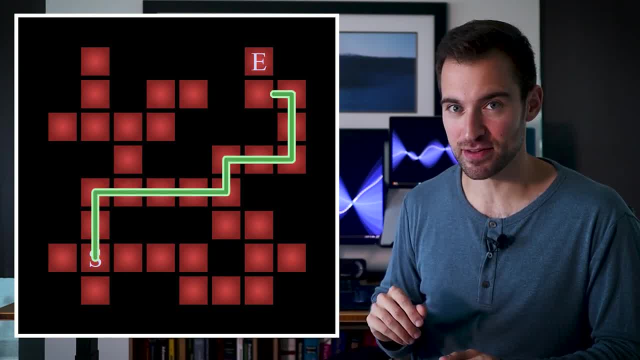 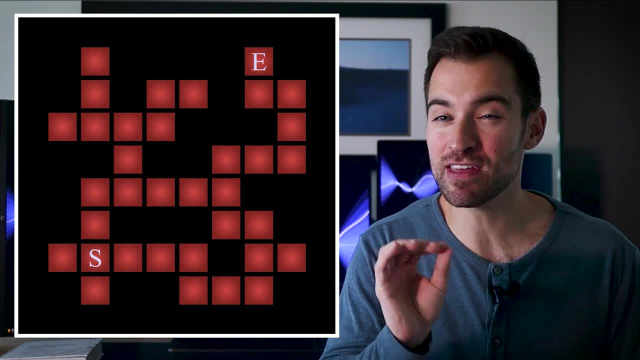 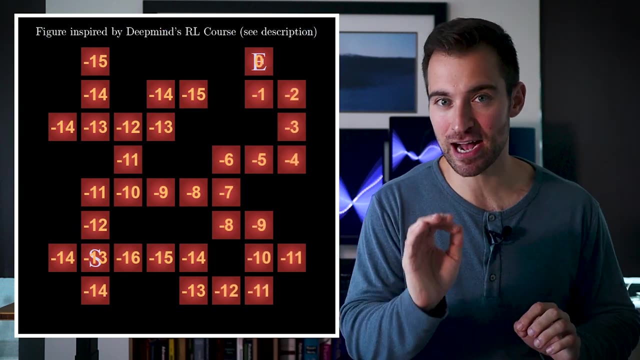 Now, because we're smarter than most mice, we can see the optimal path clearly. However, the agent can't. Instead, let's say the agent receives the state value function of the optimal policy, which will show like this: Using this, can the agent act optimally? 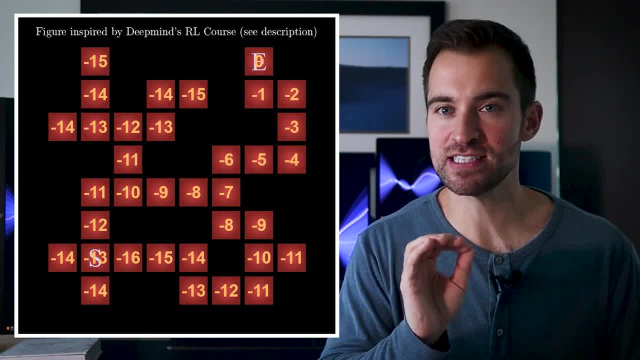 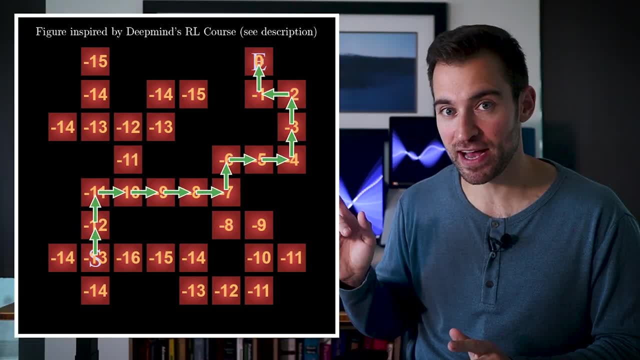 Yes, And that's the point. It only needs to follow a simple rule: Select the action that moves it to the highest value state. Doing so will move it along the optimal path. Now, this is a particularly simple example, with no randomness, but we'll handle that later. 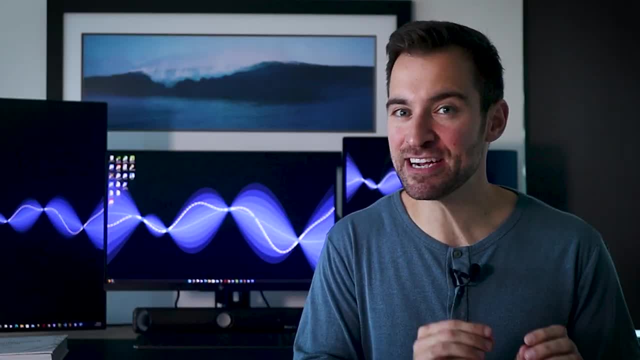 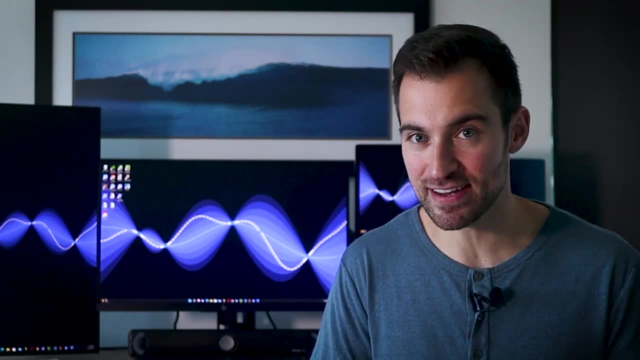 The point is the value function and, similarly, the action value function of the optimal policy provides instructions on how to behave optimally. That's the key idea. Now, to wrap up, I'd like to highlight some of the major assumptions embedded in this setup. 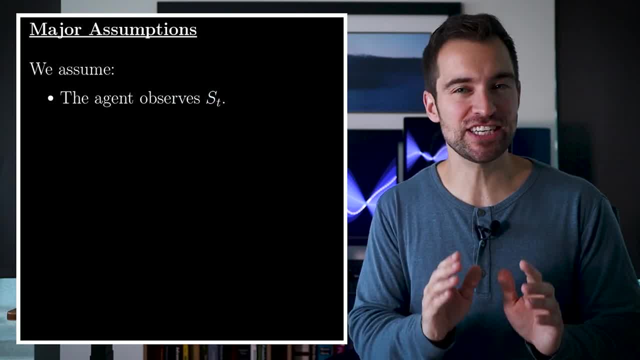 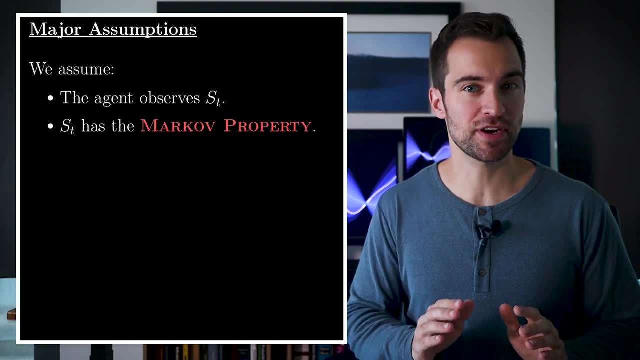 First, we assume the agent observes the state at each time step. That's a big deal. Second, we also assume the state is all you need to anticipate the future. That's what the Markov property does, and that's another big deal. 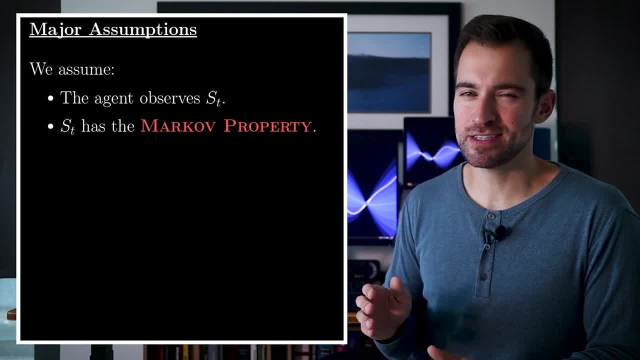 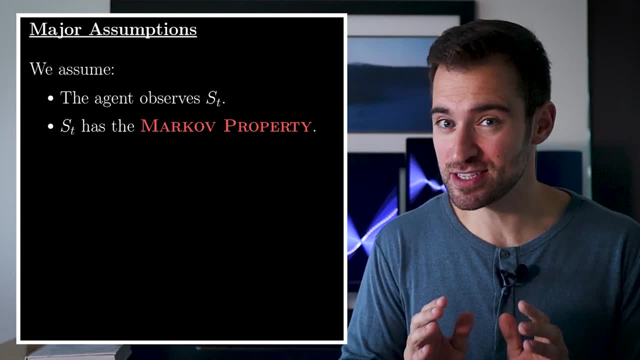 So let's back up. If you just imagine the rule, It's clear that these assumptions virtually never really hold. Just think about yourself as the agent. When making decisions, do you ever get to consult a perfectly comprehensive world state? No, You just have your limited observations and foggy memory. 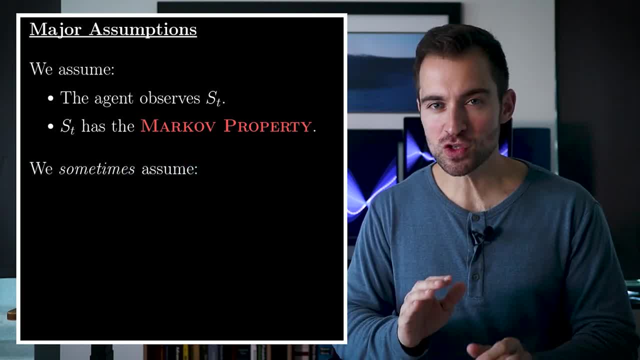 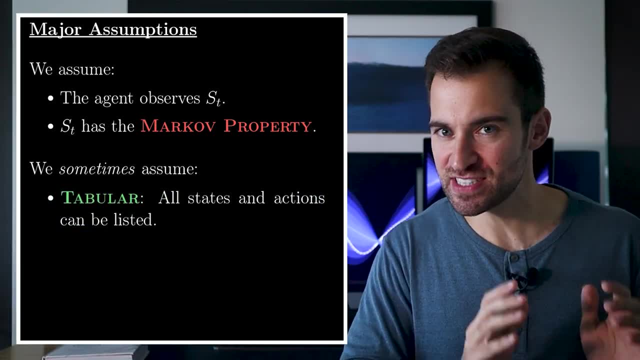 Now let's talk about assumptions. I'll be turning on and off First. we sometimes assume we can list out all possible states and actions in a table When the number of states is exponentially huge. this can't be done When it applies. 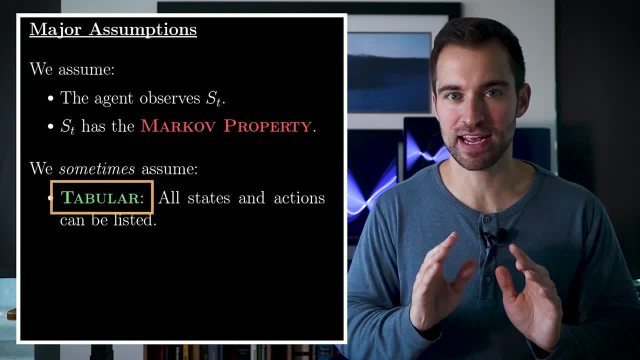 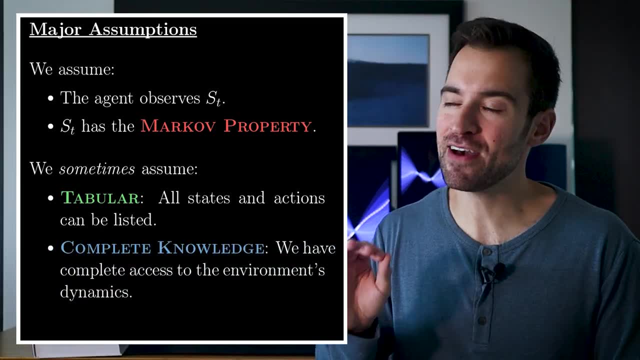 And it does up until part three. we say it's the tabular case. Finally, sometimes we assume we know the dynamics of the MDP perfectly. This may take the form of having access to the MDP's probability function. In a case like this, we say we have complete knowledge. 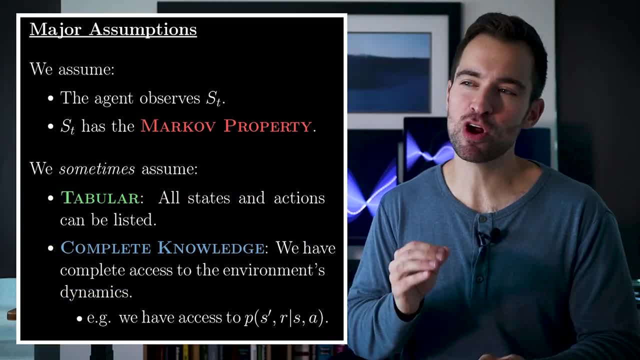 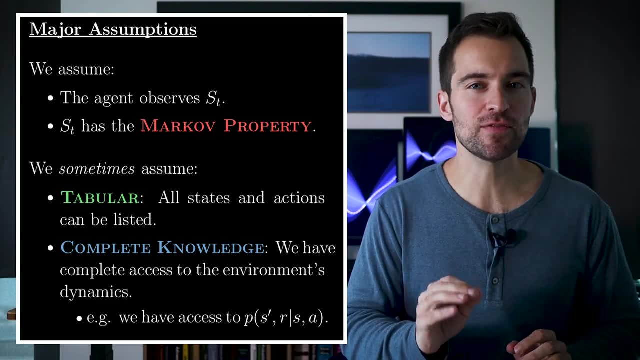 And it's an assumption- we'll start relaxing in part three. That said, the problem set up as given still serves an absolutely vital purpose. It provides the basis for powerful theory needed for the discovery of optimal policies. As these assumptions are peeled away, the theory no longer applies. 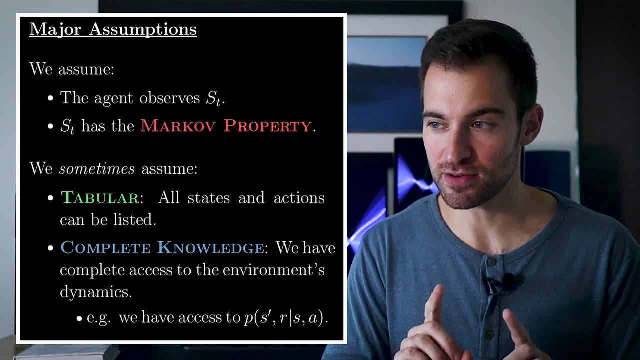 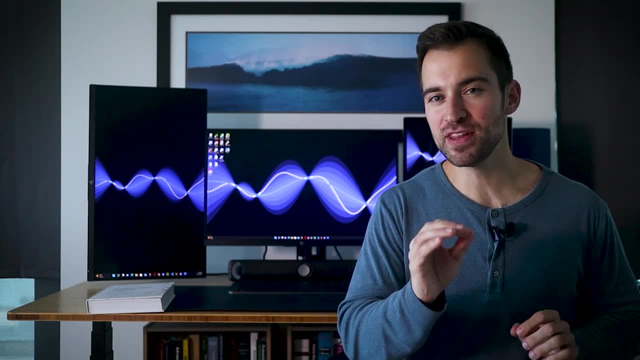 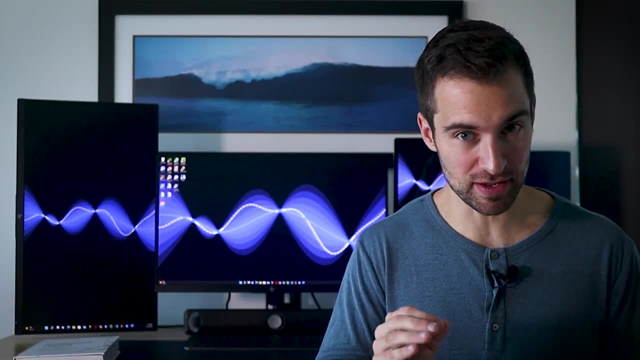 but still serves as a primary source of intuition. So it must be learned. And now the next step is to watch the next video. There you'll see how really clever and general algorithms can walk us towards a globally optimal solution. And if you're tough, ambitious and disciplined- 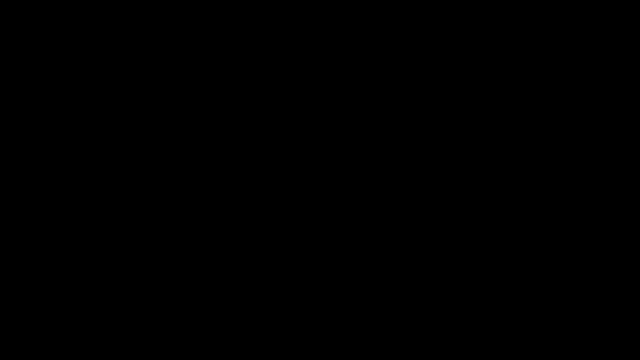 you'll watch that as well. Good luck. 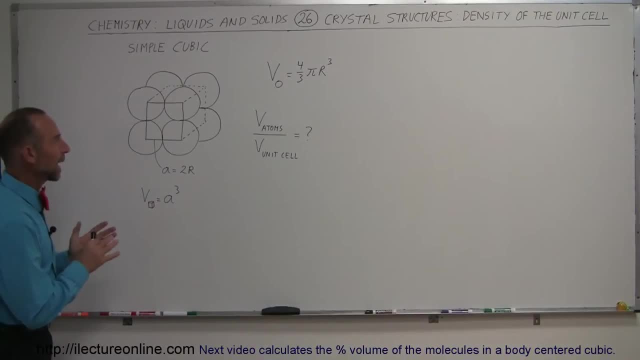 Welcome to Electron Line, and here we're going to take a look at the crystal structure of atoms packed together in what we call a simple cubic form. Now, this is not a common form. It's common in its shape, because there's many, many crystals that can be drawn out like that, where we can draw 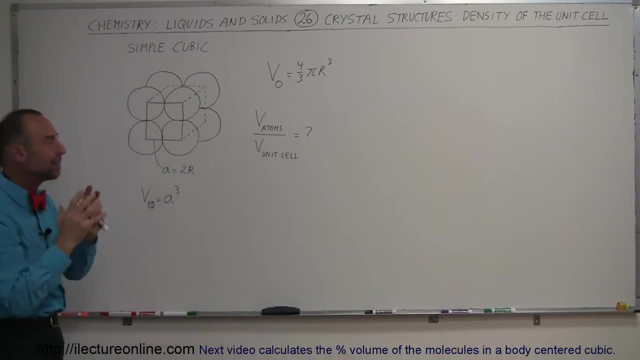 what we call a simple cube, and that cube will contain the exact same number of atoms in the same way, no matter where in the crystal structure you put that cube. But because of the electrical attraction repulsion, because of the empty spaces that are created with certain ways of packing the 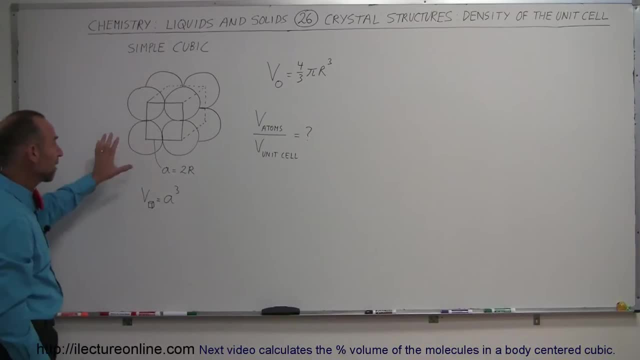 atoms. some are more common than others. Now, of course, they have a structure like this: All the atoms or all the ions will have to look exactly the same. If they're different in shape, they will look a little bit different. they'll be packed, it'll be different as well, But the object 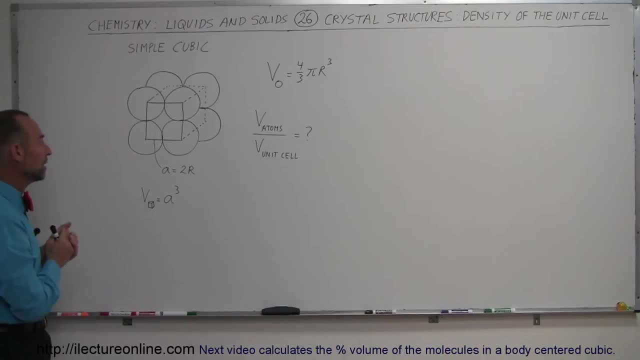 here is to take what we would call the simple cubic structure here and find out what percentage of the volume of this cube is occupied by the ions or by the atoms inside, and what percent of theどう вы咬 detail trong adsor 점? ụy面的これはどれ rico? or 답题的 wrap arranged from the atoms inside, and what percent of the. 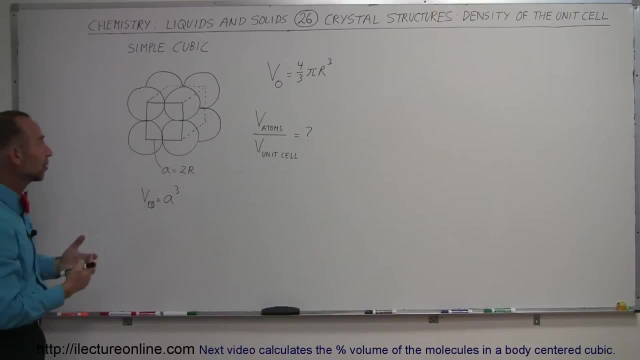 the volume. there is actually empty space where there's no atoms to be found, like the crooks and crannies, so to speak, the empty spaces between the atoms or the ions. Alright, so what we're going to do is calculate the volume of the atoms contained within this unit cell, divided by the volume of the unit cell itself. 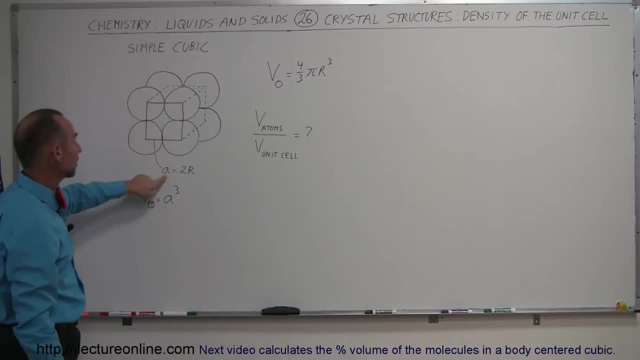 Now, if we assume that the length of each side has the value of a, in this case a would have to be equal to twice the radius of one of the atoms, because here we have one radius and here we have two radii, so the two together form one of. 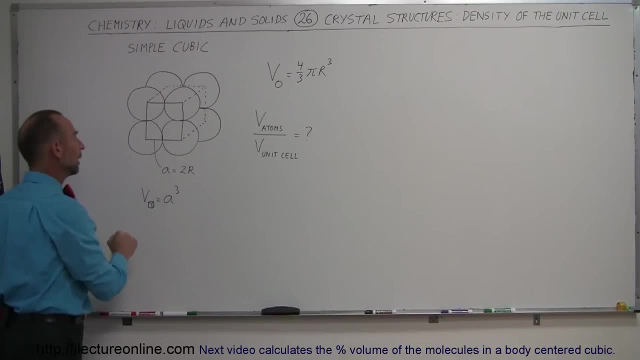 those sides, and so we know that the volume of the cube is equal to a cube, and we'll figure out in just a moment what that is equal to. We also know that if the radius of one of those ions or atoms is r, the volume of that would be four.